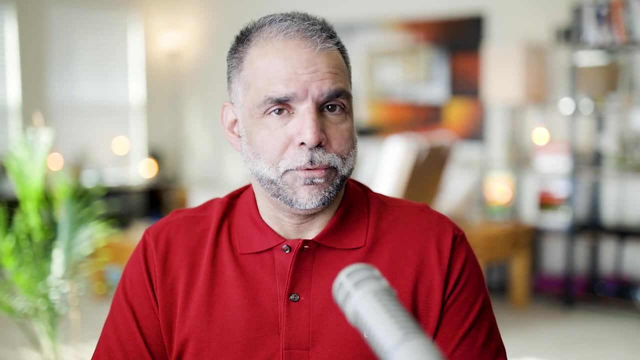 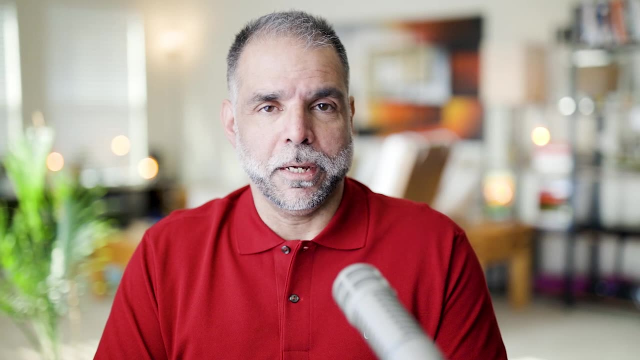 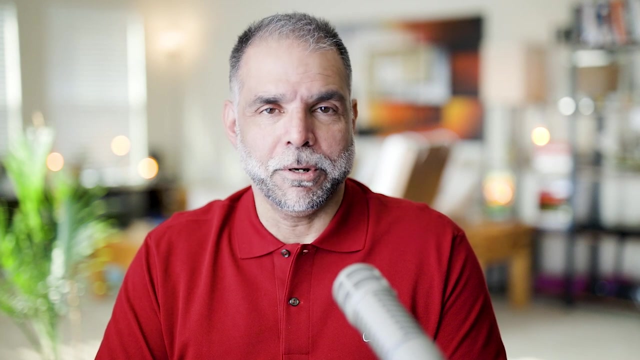 value. There's nothing much to it. There are a few popular databases or well-known- and not necessarily popular, but well-known certainly- databases that fall under this category. Amazon's Dynamo Was the one of the first databases that came out of this. this category generally just NoSQL stores. 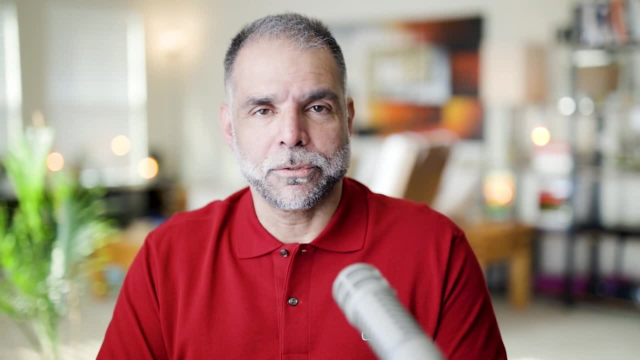 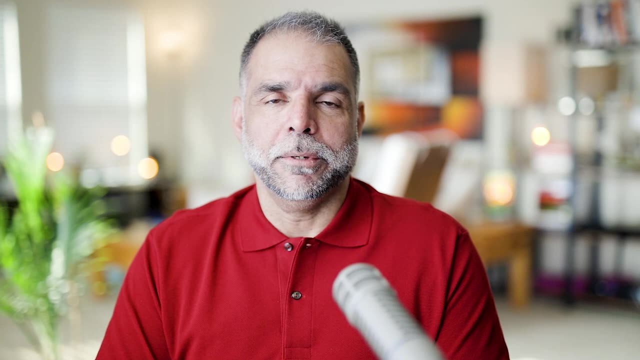 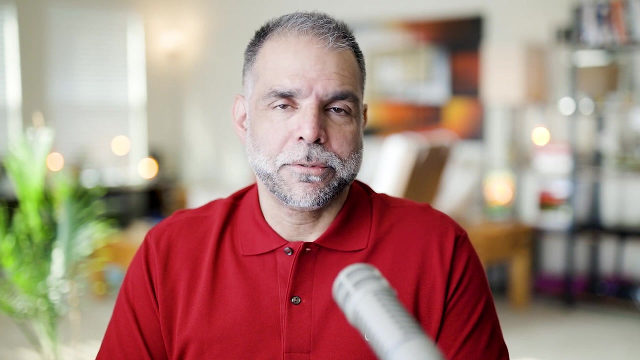 That's not to say the NoSQL idea was new at the time. It wasn't popular. It was known a few years ago. but Amazon came out with this Dynamo database that they started using for their own- not necessarily the cloud, but, you know- to run Amazon- and they published a white paper on this. 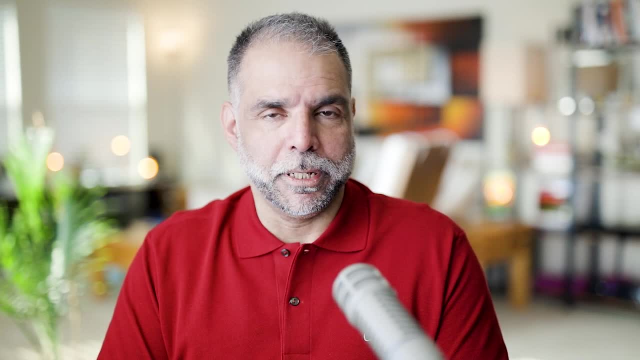 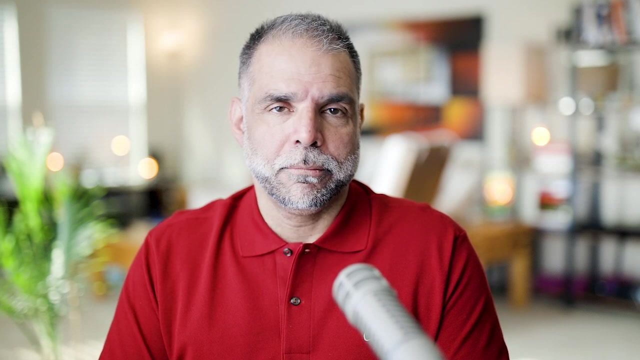 database Dynamo and many, many people picked up that white database white paper and started working on their things. Microsoft did the same. They took that white paper and they built Azure table storage as part of this idea. but Amazon Dynamo is a key value store, Redis is a key value store. React is a key value store. 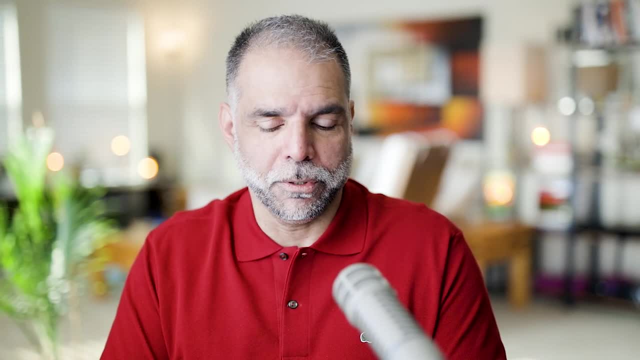 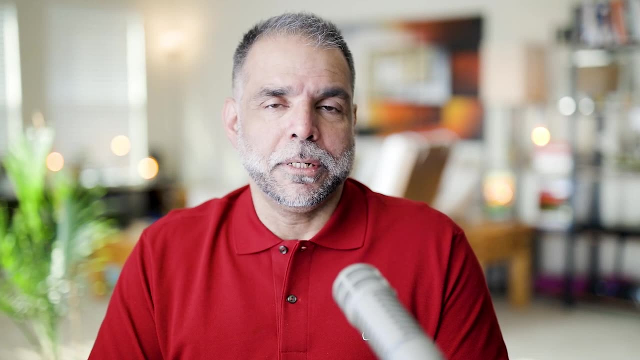 So these are examples of NoSQL stores that are key value stores. Now it so happens that Redis and are like in memory Amazon's Dynamo is not. It's an actual database that gets persisted or durable store. One could say that Redis or Redis is also durable. 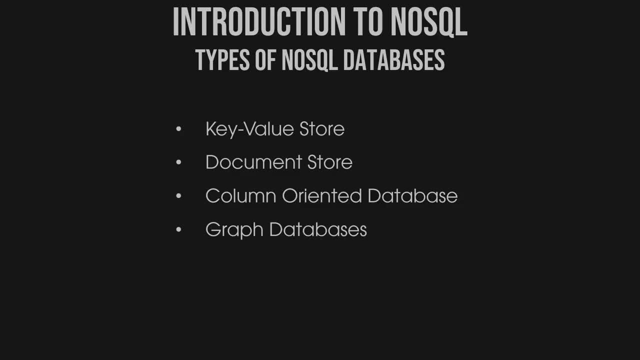 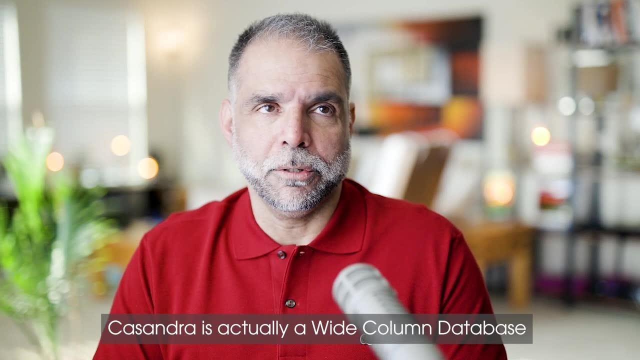 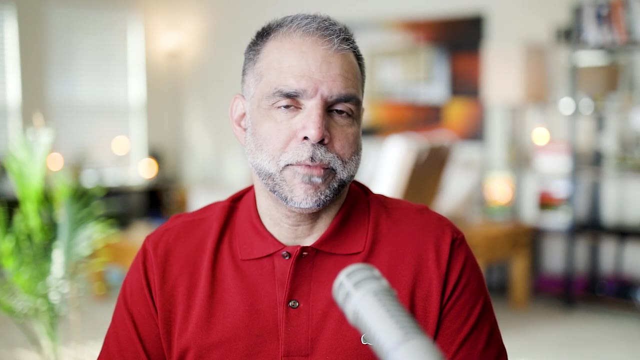 But they are key value stores. The next is document stores. Document stores are stores like MongoDB and Cassandra. Cassandra is from Facebook. MongoDB, I believe, is from the originator of DoubleClick, I'm not sure I'm mistaken. Either way, it's well known MongoDB, and so is Cassandra. 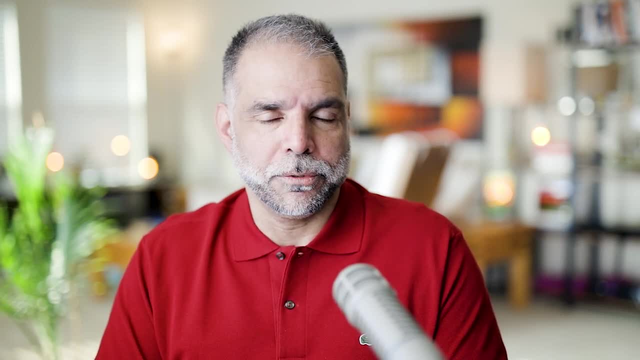 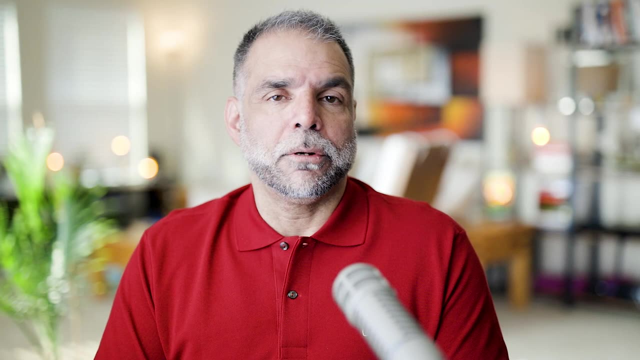 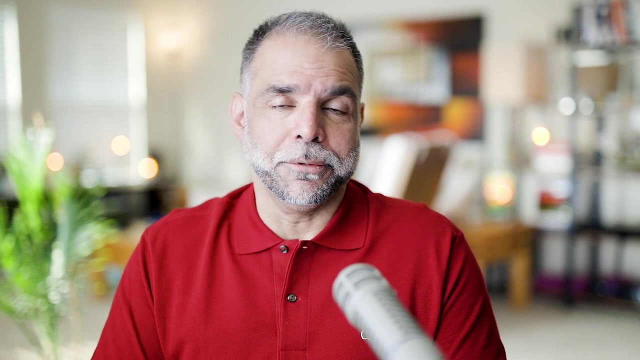 Cassandra was sort of started by Facebook. Both are open source databases, So while key value stores are a key and a value single field, generally, That's not of course true. if you look at Redis, for example, They can have a whole JSON object you know as the value part, But a document store is sort of the same thing. 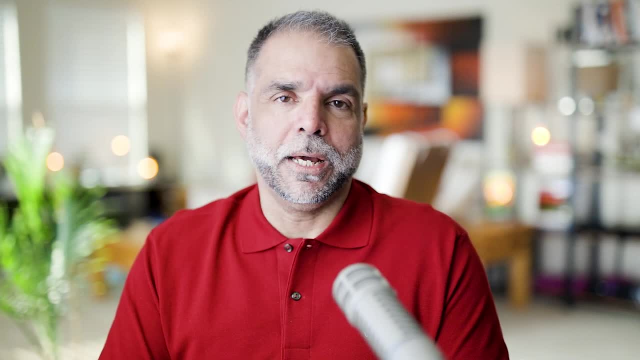 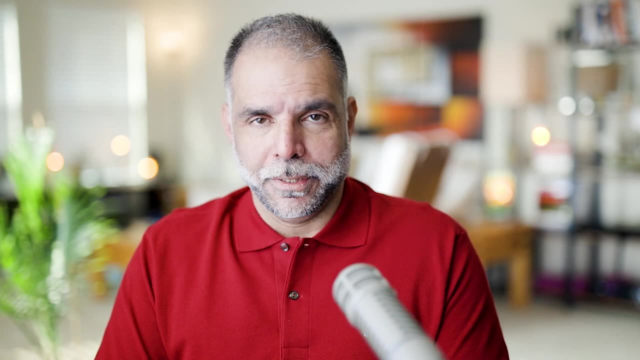 There's a key and you have to assess, be unique, and then there's a value. The value again is a document, typically a JSON document. What's really been happening over the years is these different types of databases, including RDBMSs, are all sort of converging towards a sort of a 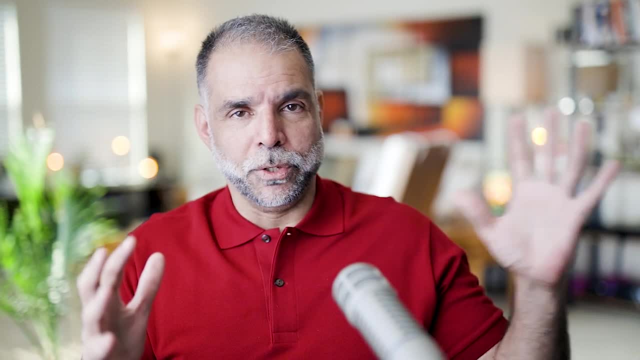 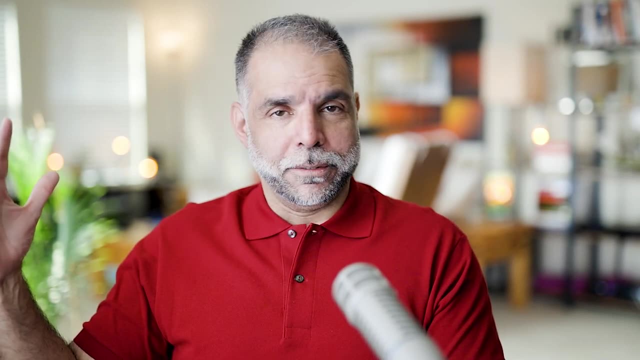 common set of features. So, while RDBMSs are doing what they do And they're trying to do some of the things that are beneficial from a NoSQL store perspective, The NoSQL folks started at a certain point. They're not only merging amongst themselves. 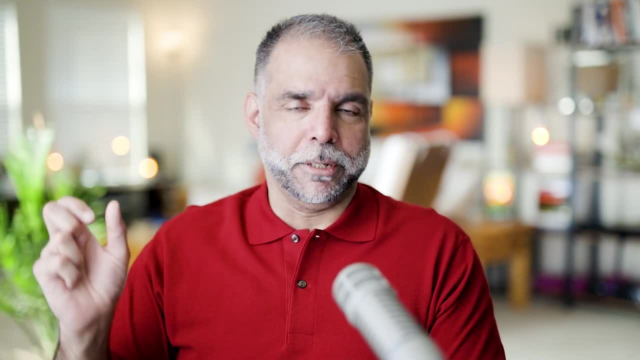 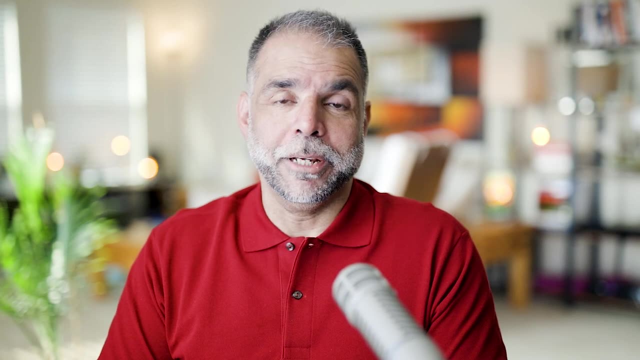 meaning their key value stores are kind of also becoming like document stores, that are also becoming like key value wide column stores, But they are also converging towards databases, right? So I think maybe you know, 10 years from now, maybe I'll be making a video that. 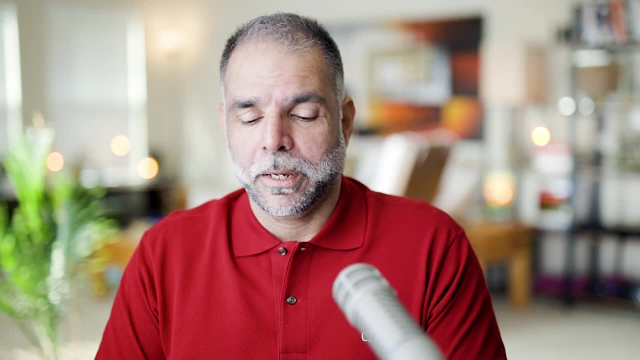 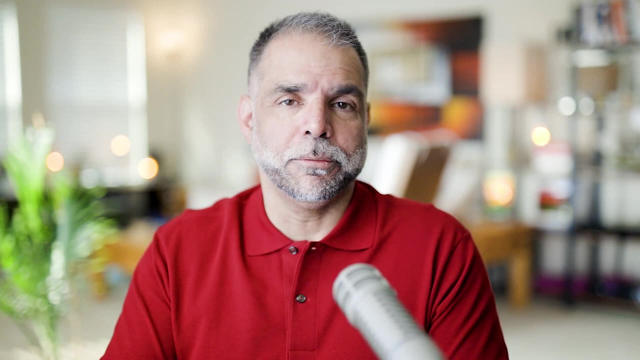 talks about how this conversion has occurred. I'm not sure, But you certainly see it from RDBMS's perspective as well as from the NoSQL store. So today I said: Cosmos DB- sorry document- stores MongoDB and Cassandra. they are nothing but key value stores. 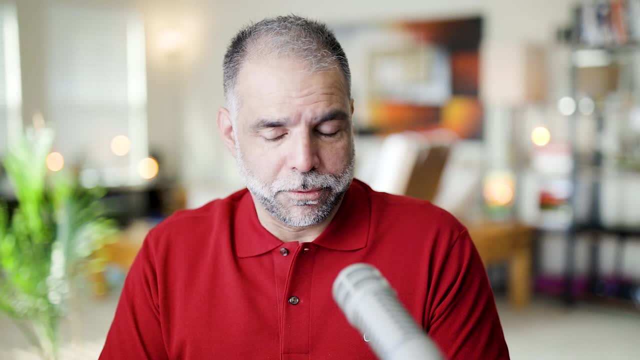 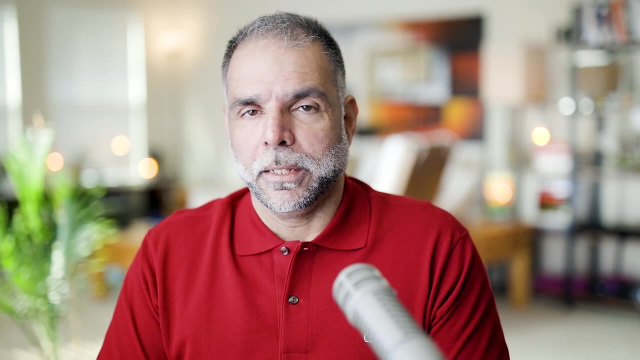 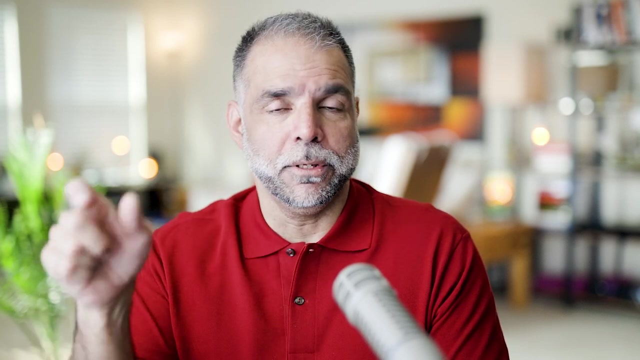 But the difference is that in document stores in this case, like MongoDB, they support Azure transactions, which is not normal for NoSQL stores, And they allow you to index fields in your JSON document. So within a JSON document you can index on certain fields including, I believe, arrays. 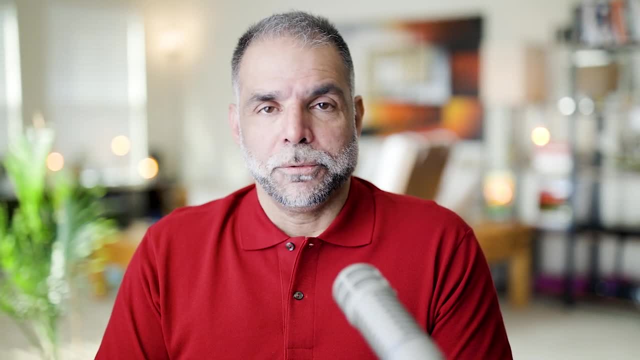 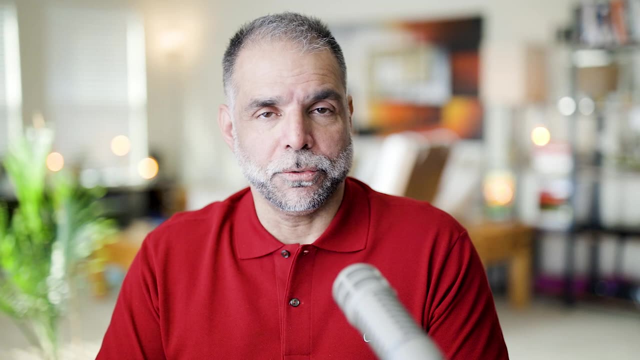 fields that are arrays And so that helps you speed up the searches right. So that's different from like in the case of key value stores, You don't, you can't index into the value part, You only have the key as an index. 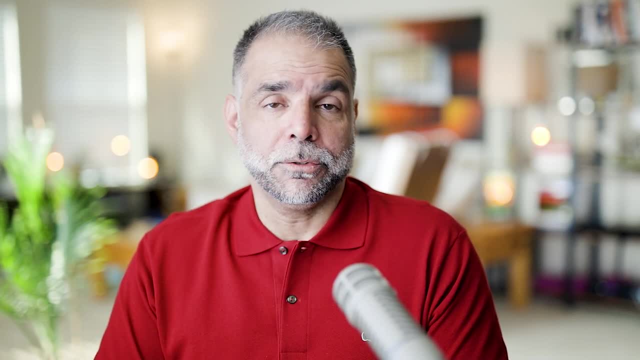 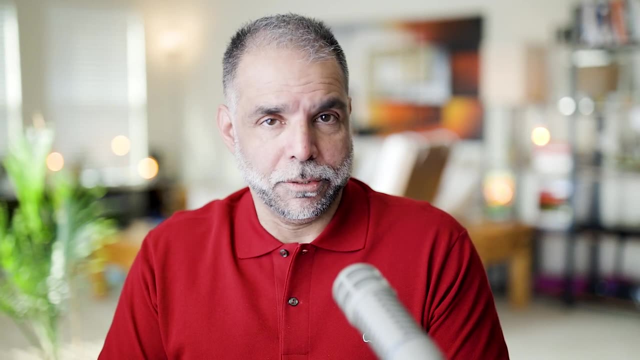 Document stores allow you for doing that as well, But there was a time when document stores didn't allow you to index into the document itself. The only index you had was the key. Now they allow you to index into the fields, and what any field you choose: Column oriented databases or white column. 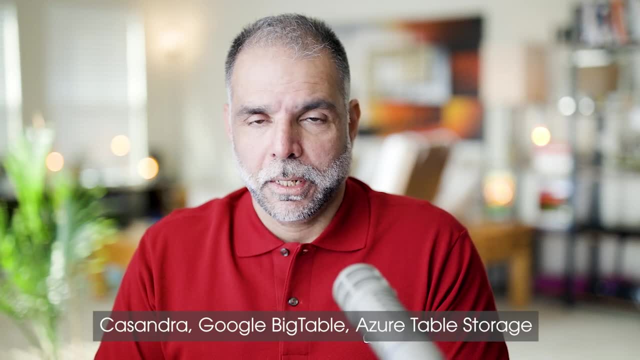 actually, they also got a lot of data. So that's a good thing, So that's a good thing, So that's a good thing, So that's a very good thing. E warnings- forоб Databases are like as your table storage. 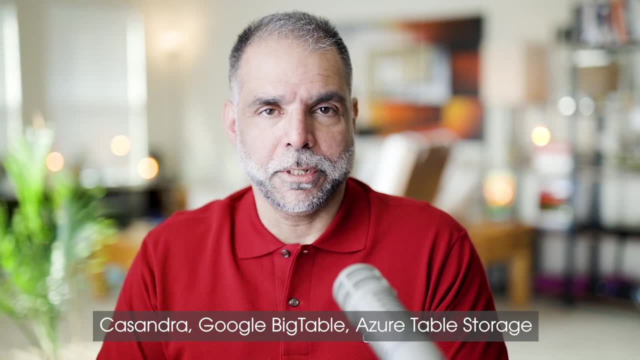 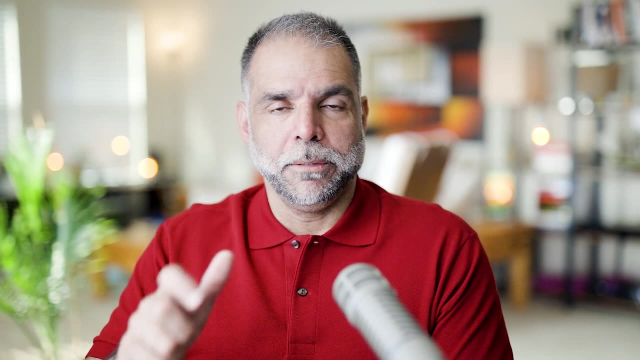 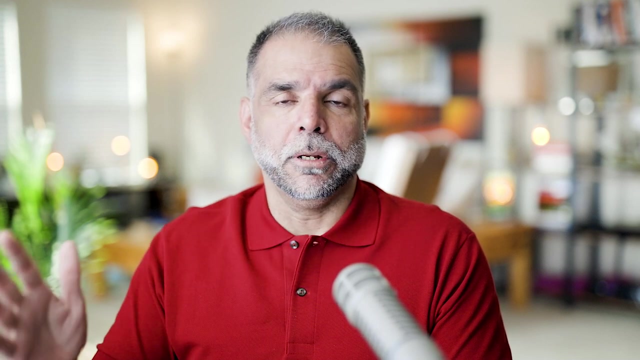 Which is it's like a table- RDBMS Table- where you got a key and columns n number of columns. The columns have no schema. is this name, but there's noيتhe following ing the data, Other names? just there's no data type, but for the column it's just column. 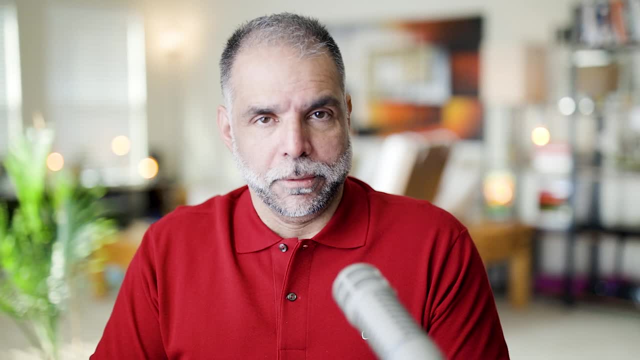 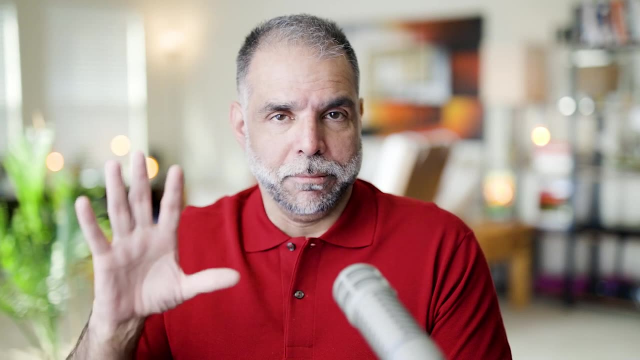 So if you can put whatever you want in these columns and one of the what I would say benefits of In this context, there's no easyně how annoyance with data typically in this hold NoSQL stores is. they are schemaless, which basically means that the next row in the same 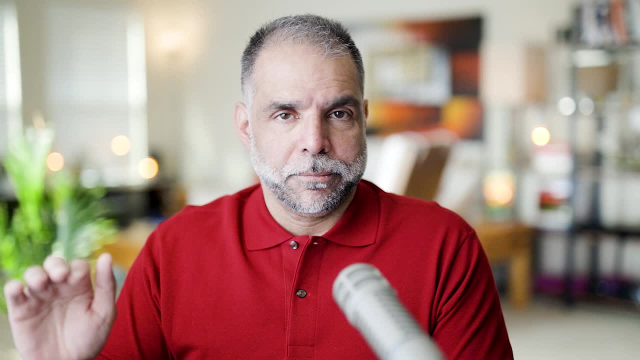 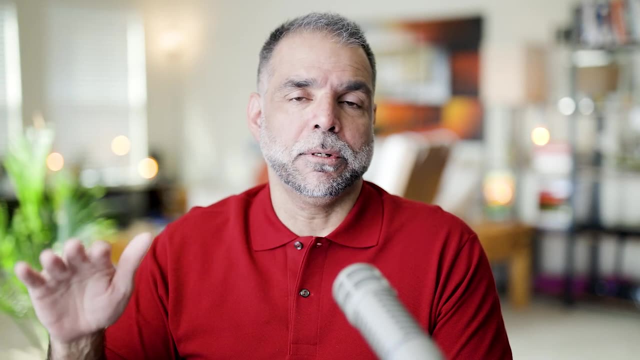 table can have completely different data, not even the same set of columns. So if you were to look at them in a tabular fashion, you might find gaps in certain places. for the next record, not because there's no data, it's that the schema itself is different. 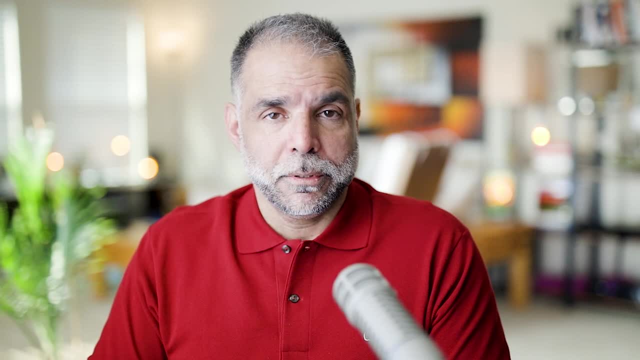 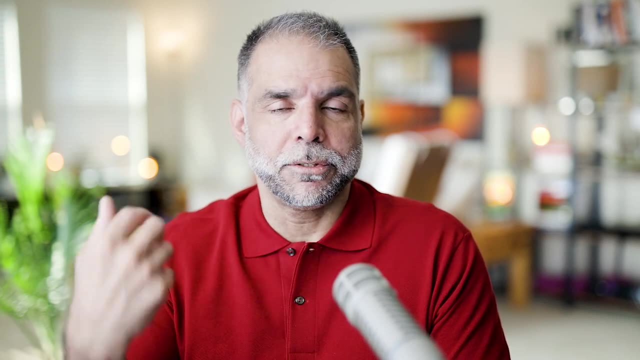 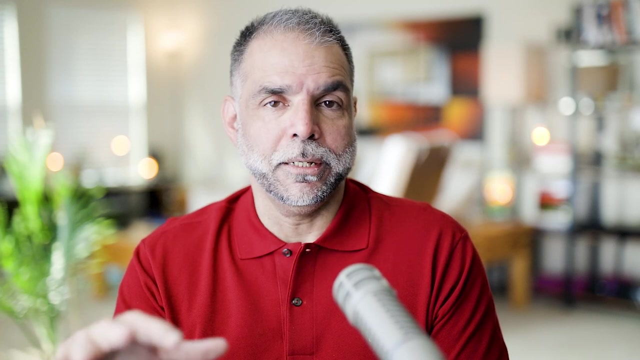 So white column data stores allow you to have multiple columns, still only one index and every record could potentially be a different schema, The schemas in your head. it's not like you set it up in the NoSQL store itself. The containers or the tables don't have the idea of a schema, but of course in your application. 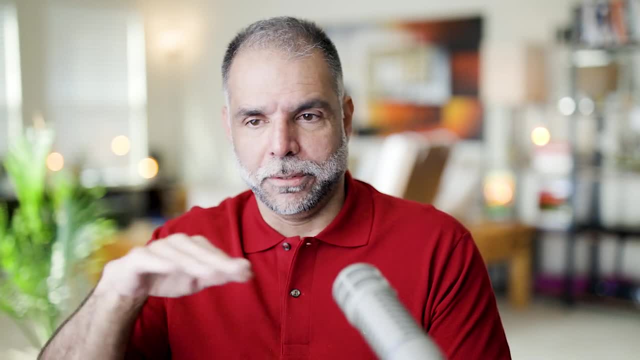 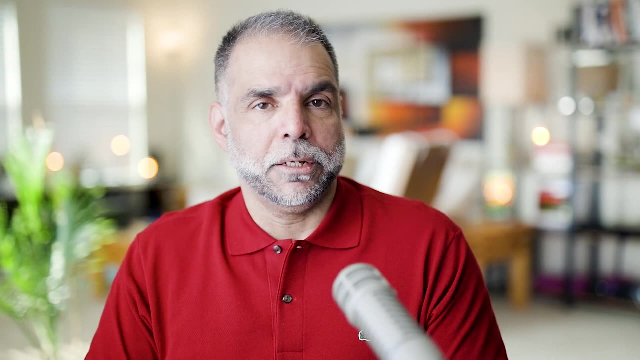 you may have the notion that this record has this schema and this next record has got the schema, So you can have different schemas for every record in these tables and you can index on the one field. and that might seem really weird. why would you want to do that? 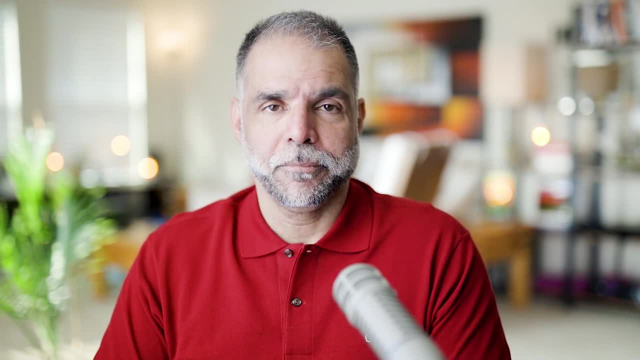 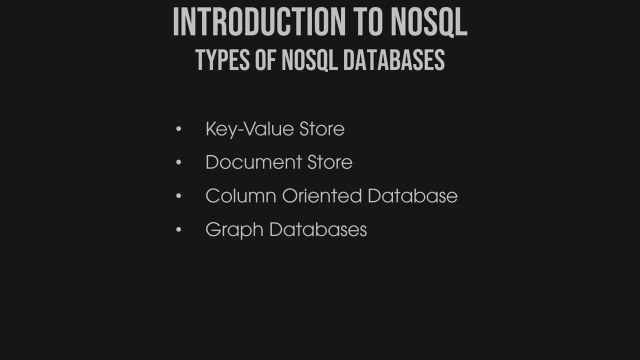 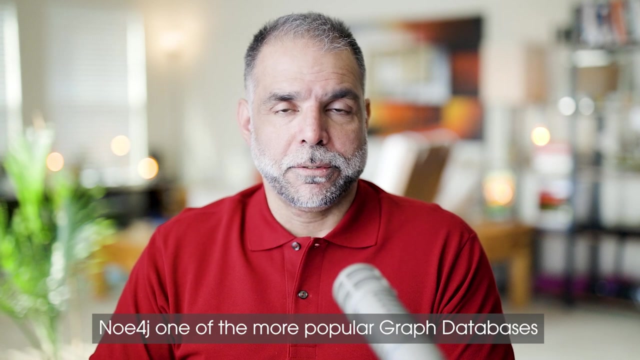 But there are advantages to having that feature or that capability And as a result of which you might want to use a white column store rather than a key value store or a document database. Graph databases are actually apart from the rest, even though they come under the NoSQL. 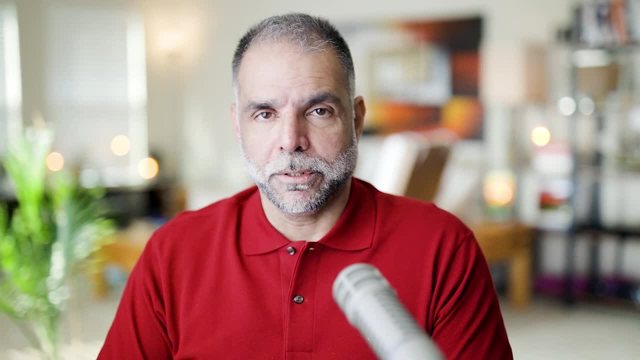 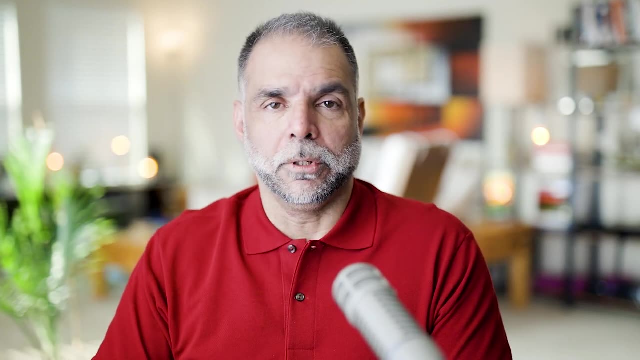 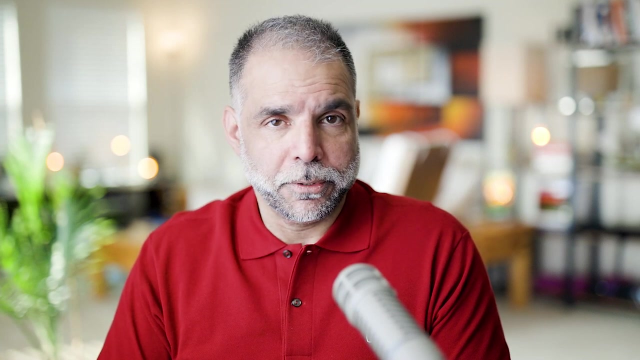 store umbrella. they are very specialized. They are very tailor-made and specialized for the notion of graphs, which is like a tree structure, if you will, not a graph as in bar chart. But they base their So engine on what they call graph theory, which is a field of mathematics essentially. 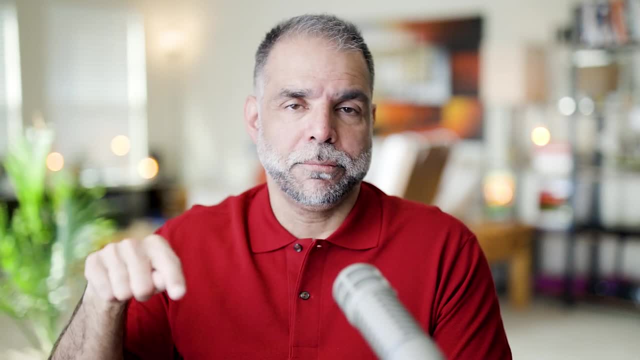 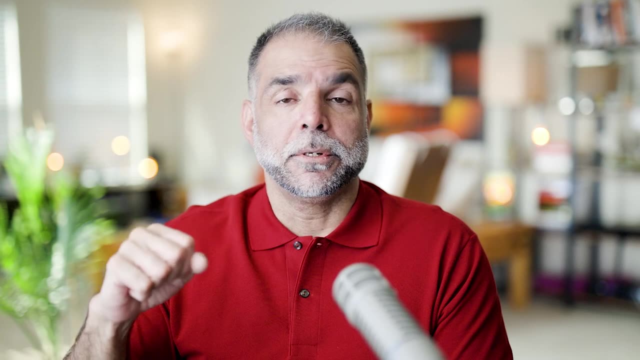 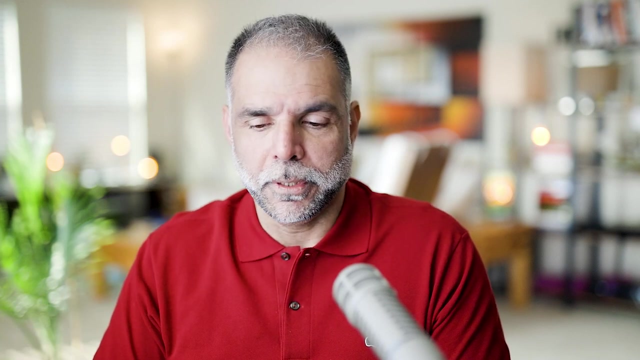 a vertices and vertices have edges that are sort of the joints between the vertices. but they can have multiple vertices between two nodes or vertices, multiple edges. So the mathematical terminology is node, vertices and edges and database terminology they call them nodes and relationships. 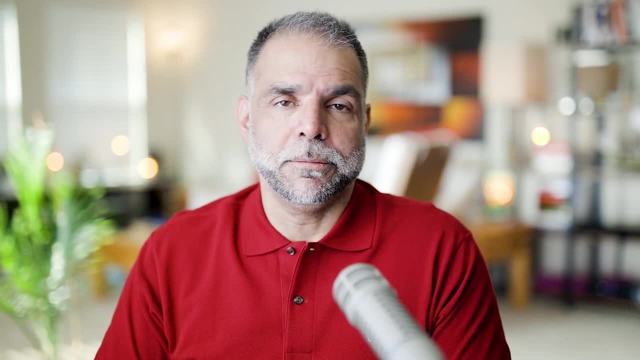 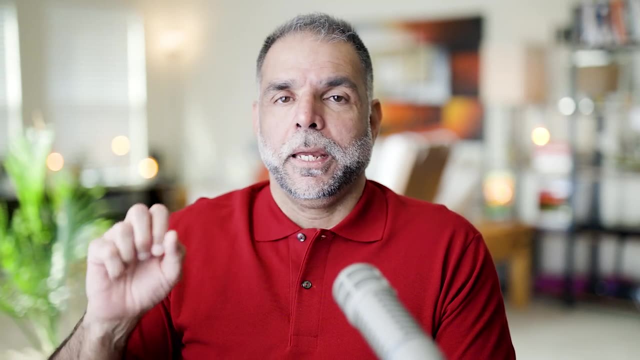 So these are directed graphs, which means the relationships are also directional. So A might relate to B, A being one node, B being another node in a certain relationship. let's say, you know, A is married to B, right? 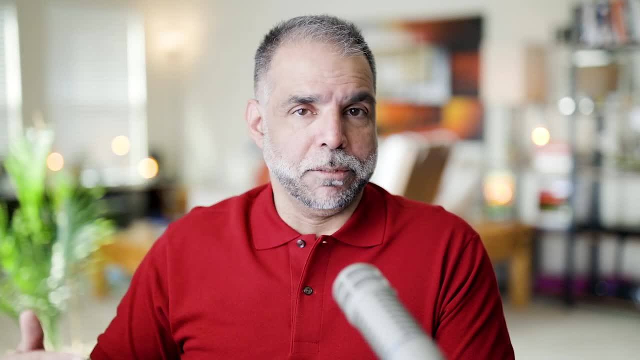 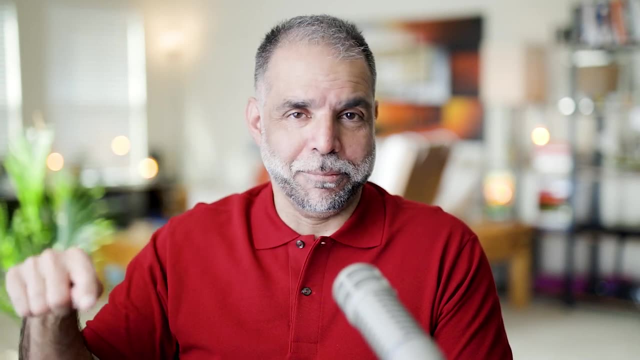 There could be a relation going backwards, meaning B is married to A right, And there could be another relationship between A and B that says A loves B and there could be another relationship from B to A that says B does not love A. just to give you an idea. 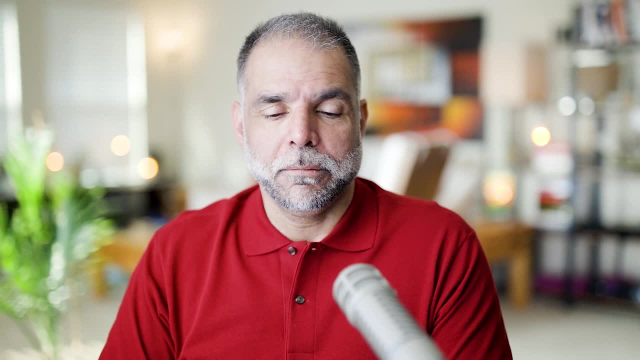 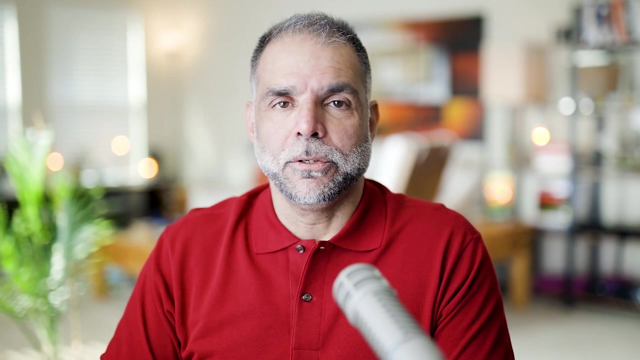 So they're directed graphs And there are many, many use cases. There are many use cases for graph databases where they give you insight into your data that you couldn't have even imagined. because of the visualization that you get with all these relationships, You're starting to see connections, maybe two, three degrees of separation from where 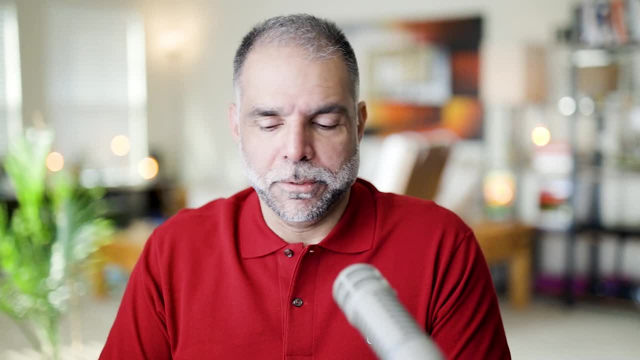 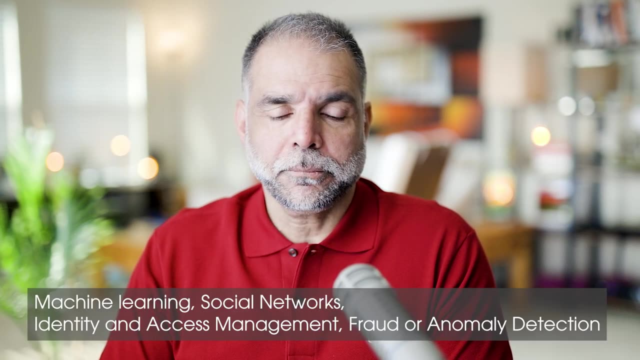 you start that you would never be able to see in an RDBMS. So graph databases have a specialized use case If you're looking at like fraud detection. if you're looking at some people talk about recommendation engines. I don't know. 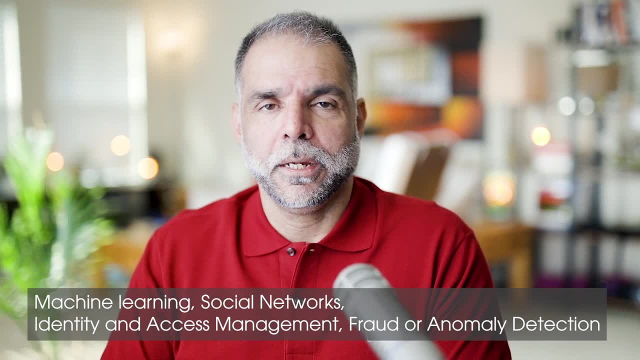 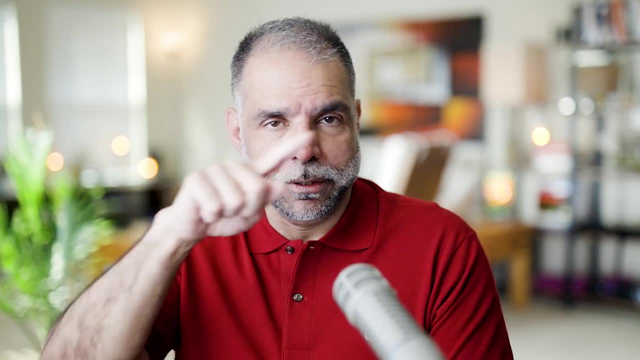 I'm not sure that recommendation engines are necessarily graph database related, but certainly if you look at LinkedIn, you know where they say: Hey, do you know this person? The way they're recommending? that is certainly because of the relationships, like you know. 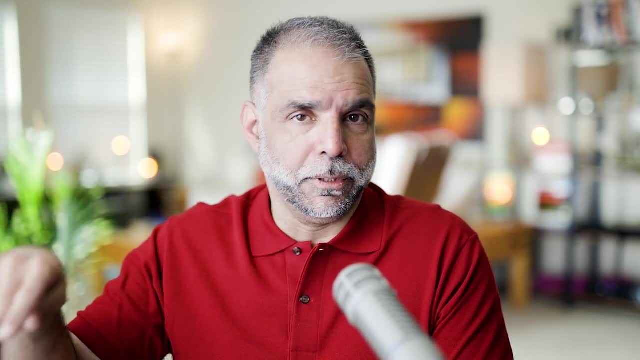 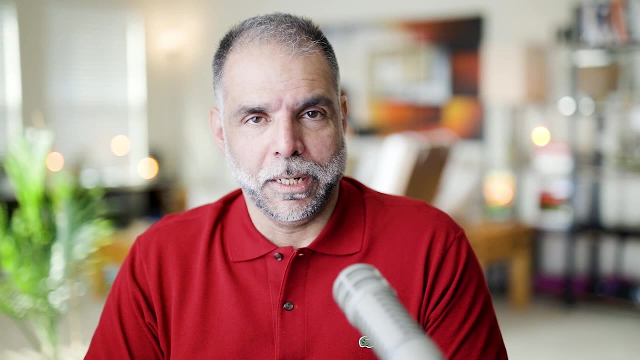 somebody else knows somebody else. therefore, you might know this person who's three degrees of separation from you And they use those algorithms to get there, but they're a specialized case. I don't think they'll ever converge into the other NoSQL stores like the document databases. 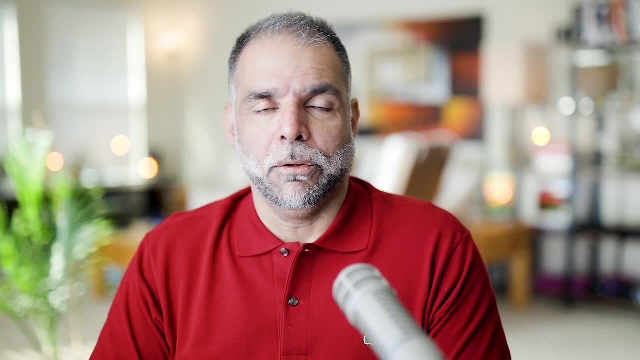 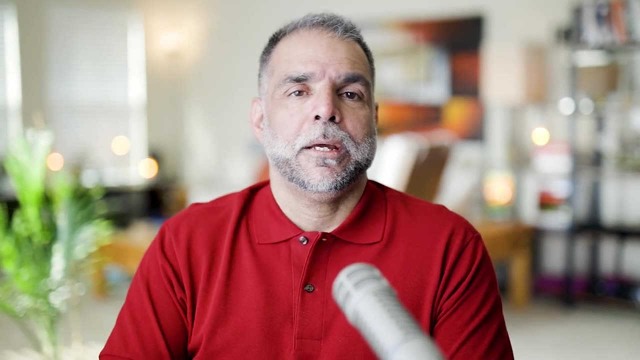 and the key value stores and the white column stores. I think they'll always be there. I think they'll always remain separate, with a very specialized use case for that. We don't want to be looking at graph databases today at all. All right, 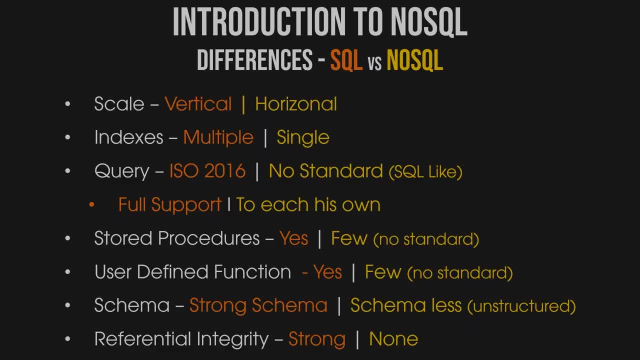 So what is the difference between SQL and NoSQL? So just to be clear here, all the SQL virtues of features are in orange and the NoSQL virtues of features are in yellow. All right, So let's look at scale. We know that RDBMS is scale vertically. 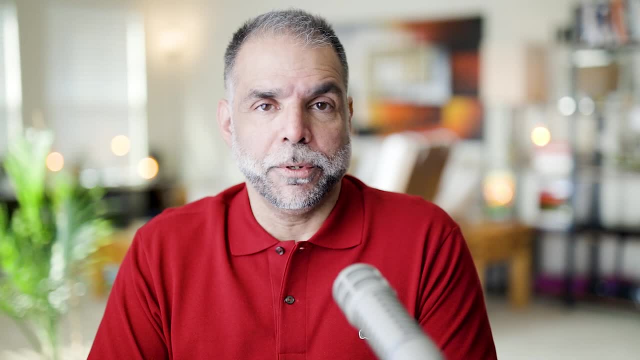 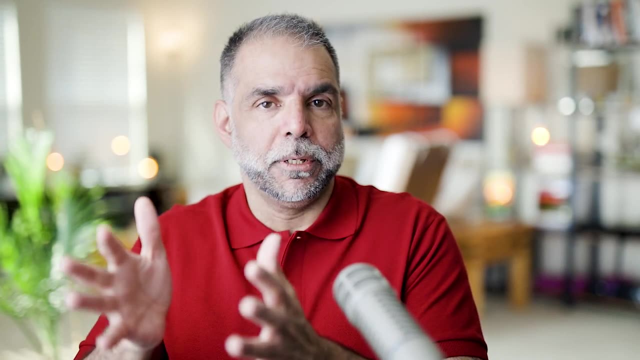 What does that mean? It means as you want to support more and more requests. So if you want to support more and more requests per second, you've got to buy more hardware. You're scaling vertically. The same machine has to become bigger and bigger in terms of CPU memory, hardware space. And there obviously comes a point where either it becomes way too expensive to keep buying more machine, more hardware, or you hit a limit right Now. there was a time in the cloud where you couldn't buy or rent large hardware in the cloud. 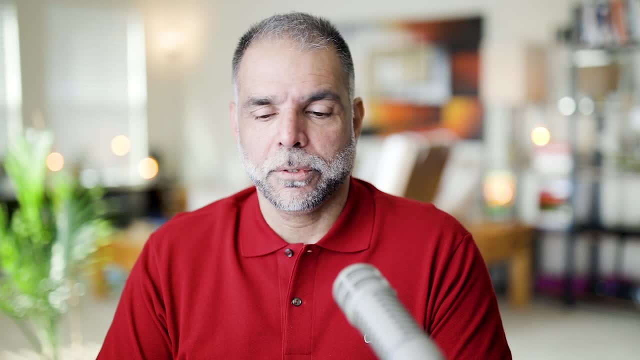 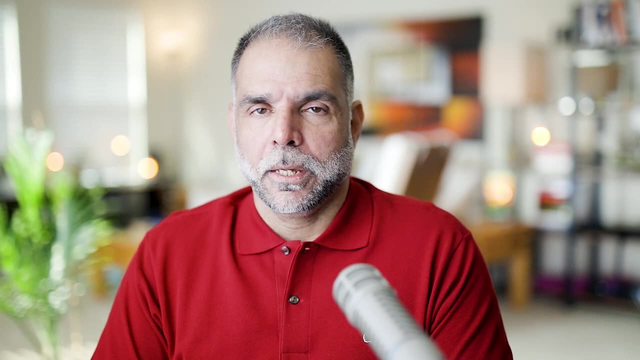 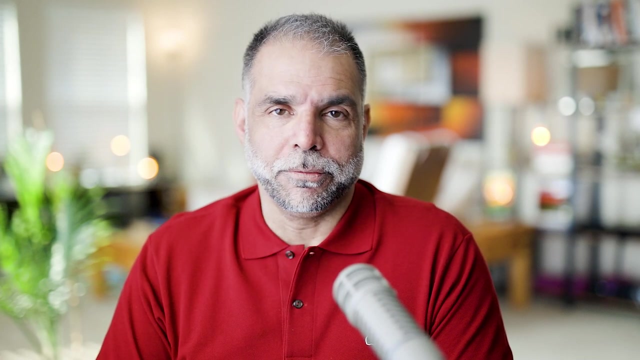 So you were almost certainly forced into using NoSQL stores if you moved to the cloud. These days, I believe, Azure supports. I think they call them the MV2, I'm guessing M stands for monster version two, and it supports like 12 terabytes of memory and 416 CPU cores, and 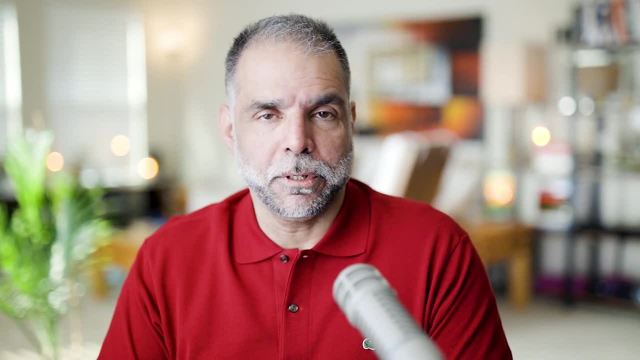 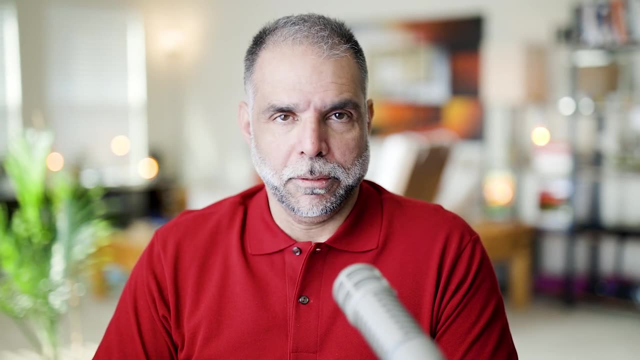 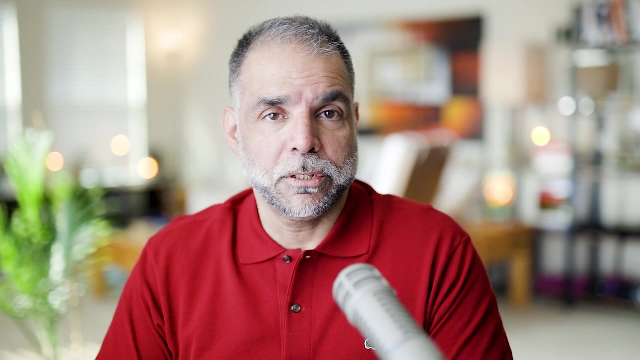 unlimited hard drives like this space, And these are all SSDs, so they're not spindles. So today, I'm not sure that that's the only none of these machines- this one I talked about, MV2, I think, would cost you about $16,500 a month just for the machine, right? Then of course the ingress and egress, as in data going in and out, all that's going to cost you additionally but that just having the machine up and running is going to cost you $16,500 a month. And of course you know, for a large enterprise you have that large data set and you need that performance? Yeah, You get one of those machines and you literally don't have to make a change. Yeah, You can just go to the cloud. If you have a machine that has a lot of memory, you can go to the cloud. 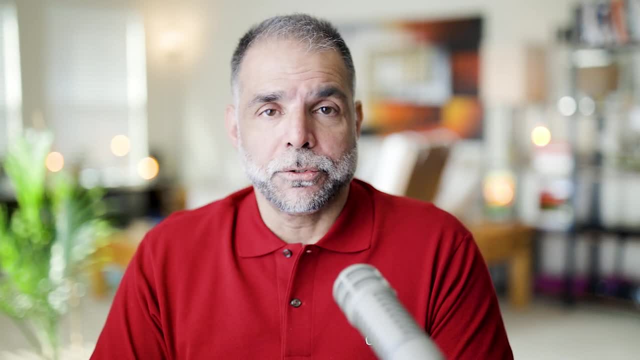 If you have a machine that has a lot of memory, you can go to the cloud. If you have a machine that has a lot of memory, you can go to the cloud. No SQL stores. So that is a vertical scale, right. 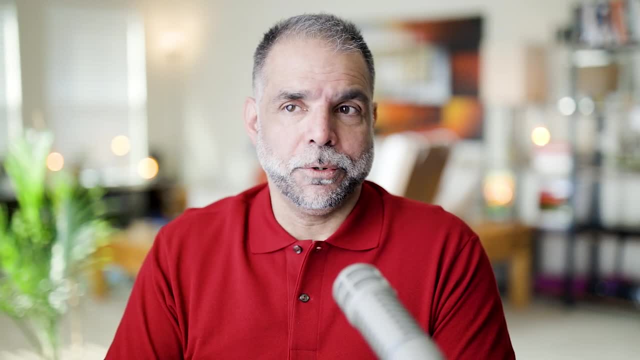 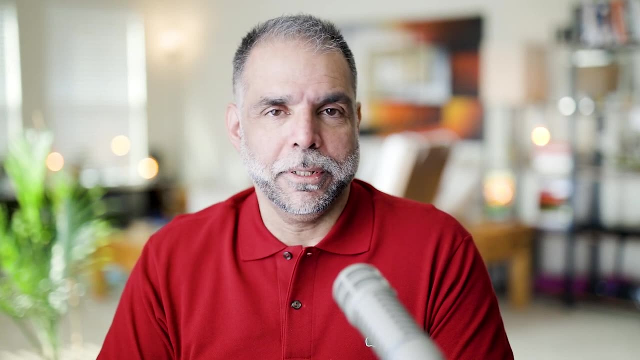 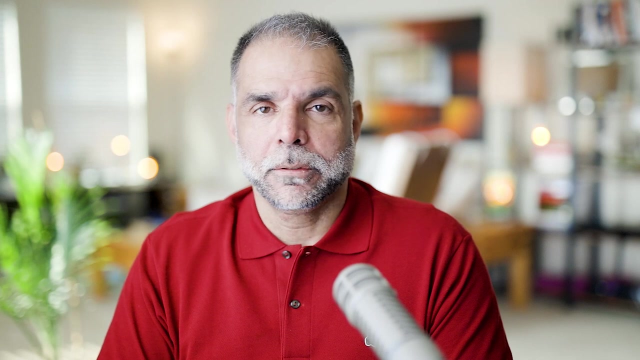 When you have a machine that has 416 cores and can have 12 terabytes of memory RAM and unlimited hard drives. this space, that's vertical scaling for an RDBMS. Nothing wrong with it, You know. some enterprises just prefer to stick with RDBMSs because RDBMSs have certain 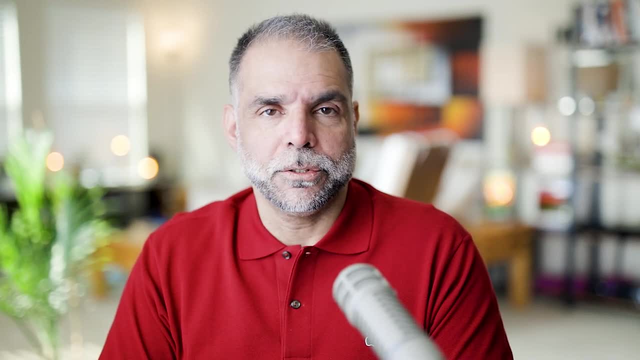 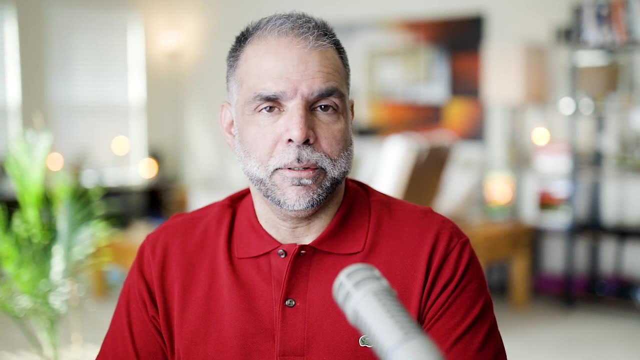 features that NoSQL stores don't. So it's not like you: you can just because you have this business or this kind of data. you can only just go to a NoSQL store, and vice versa. There are some scenarios that are more beneficial to NoSQL stores and some that have been more. 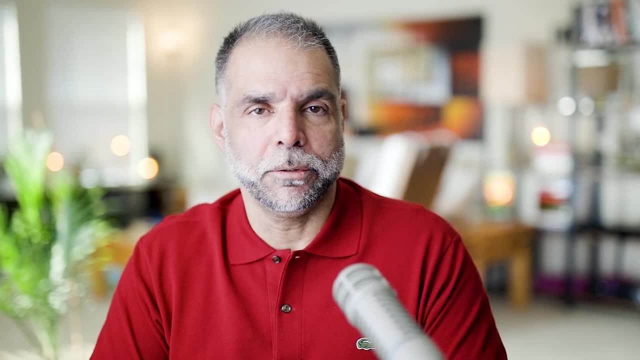 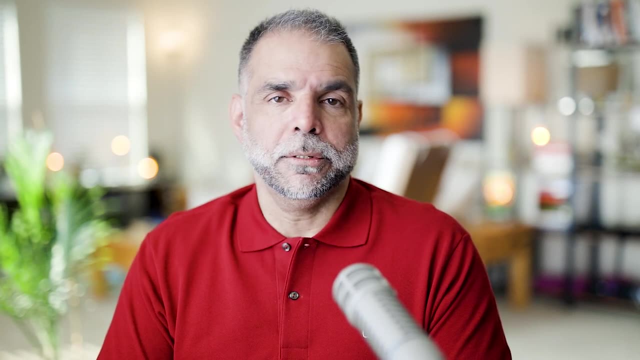 beneficial to RDBMSs and some are. you know, in between, and you can do it either ways, And because of your existing skillset and existing investments that you might have in software, you might decide to stick to RDBMSs. 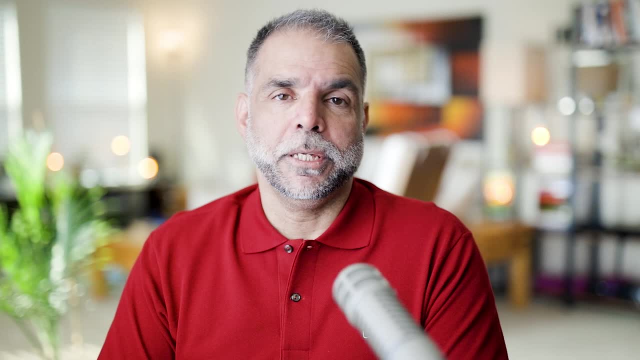 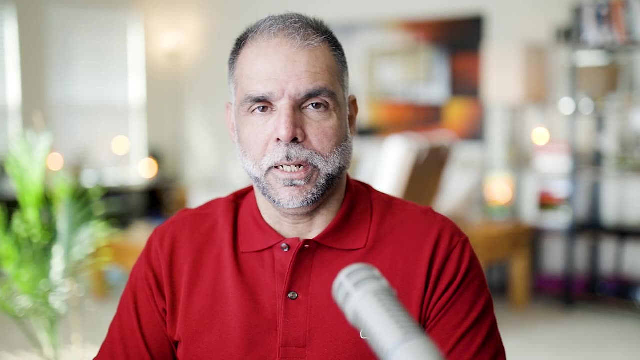 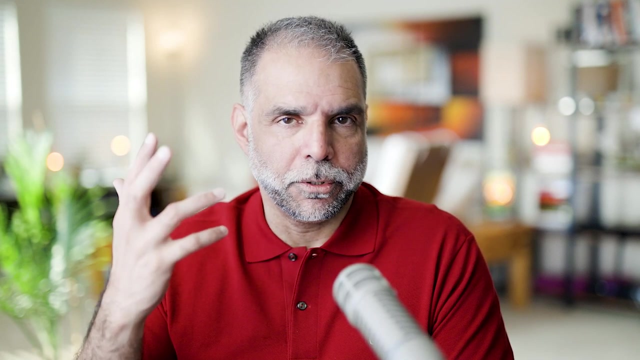 NoSQL stores are built from the ground up. They're built from the ground up to be horizontally scalable. What that means is every node, every machine, this, you know, part of the scale. scale out. Think of it as a small commodity. hardware, you know, just as an example, to put a visual, 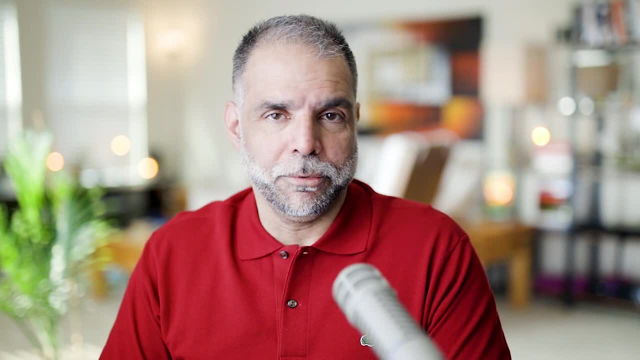 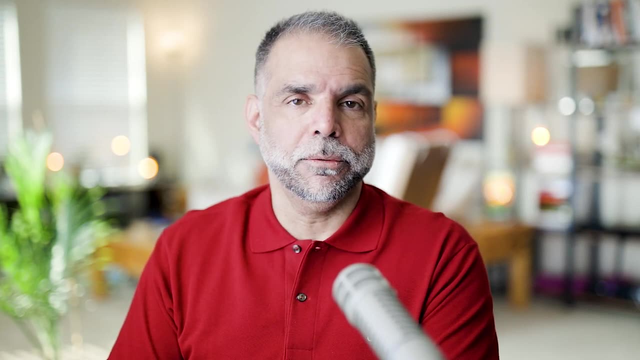 in your head- Not that that's true, but think of it as you know: your laptop, your desktop, And there's hundreds of these machines that can support your database, but each machine can only support a certain amount of load, right. 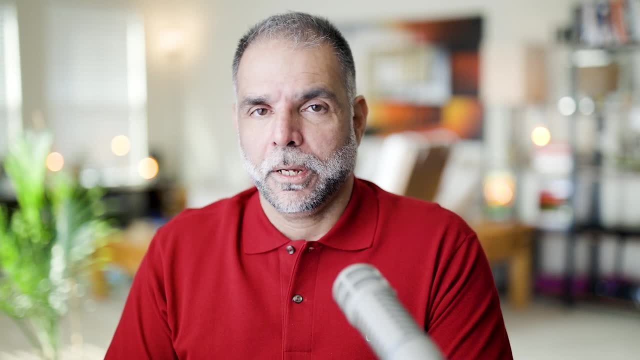 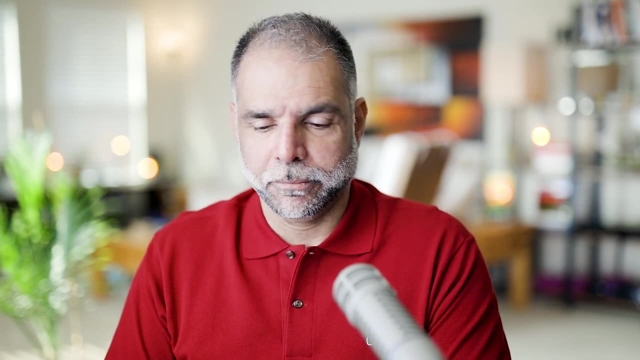 So it's not like every machine can support a terabyte of data. So, yeah, Yeah, It's not about the data, it's about the CPU power and the IO you know required to process that much data. So when you scale horizontally, you're really saying that. look a couple of things. one: 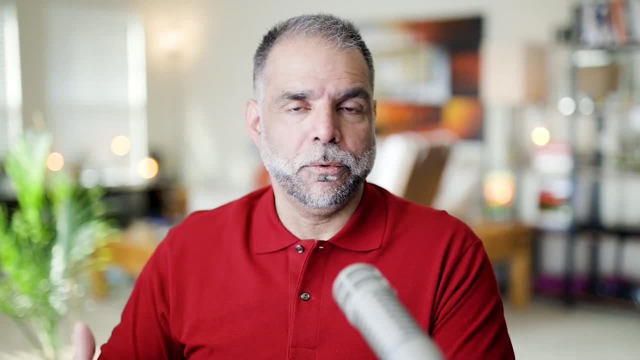 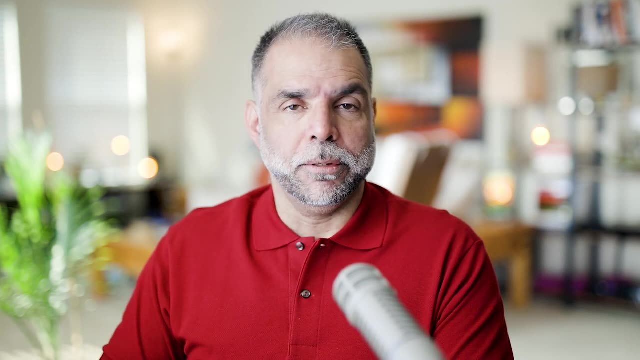 the hardware you require. it doesn't need to be this beefy hardware You don't need, you know, 416 CPU cores with 12 terabytes of RAM. They can be smaller, harder, thus cheaper. You need plenty of them to support that ability to hold so much of data and to be able to 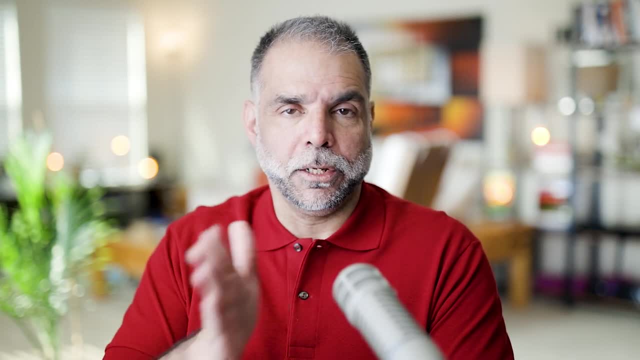 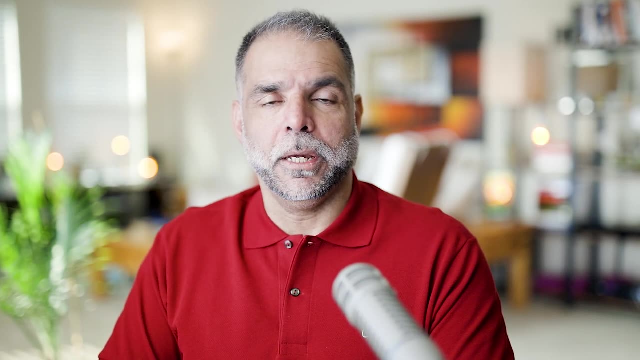 scale or handle so many requests per second, with the idea that the requests are distributed And the workload is distributed evenly, hopefully, across these shards or these nodes. If you haven't seen my database sharding video, please take a look at it here. 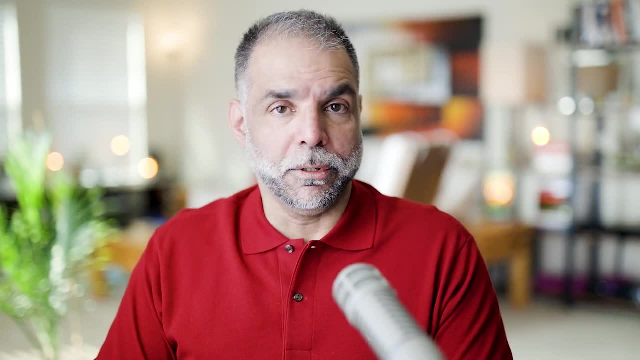 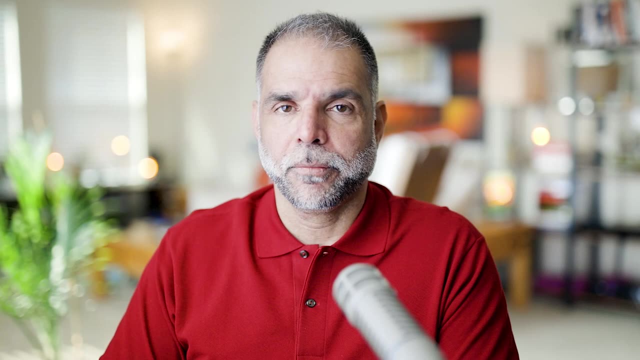 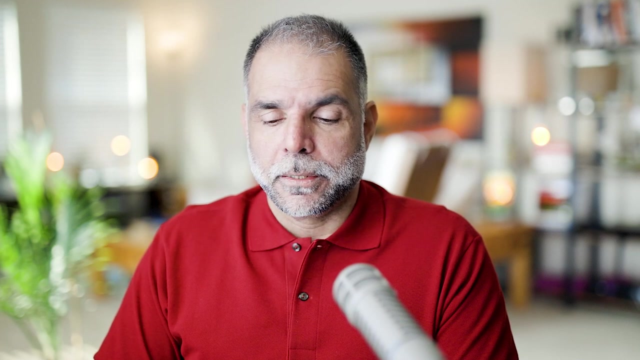 That might be useful in the from the perspective of horizontal scaling. of course, we are talking about NoSQL stores here, not RDPMSs, but it's the similar idea that applies to NoSQL stores, The sharding, if you want to call it that, in NoSQL stores, or the horizontal scale out. 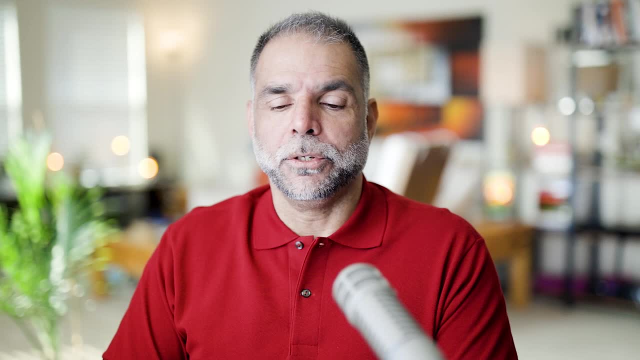 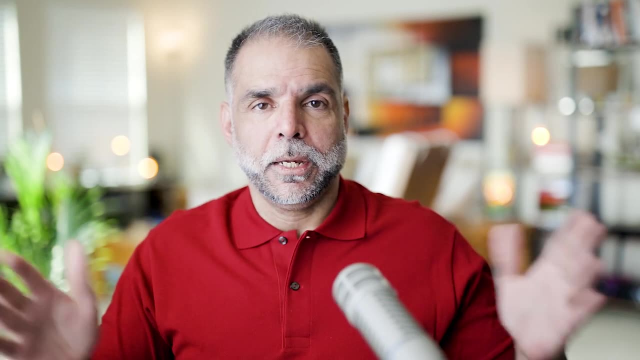 is automatic. You're not dealing with it yourselves, but you are specifying the, what they call the partition key. The partition is that partitioning like. you know what's the. why would this data go to this machine And why would this data go to that machine? 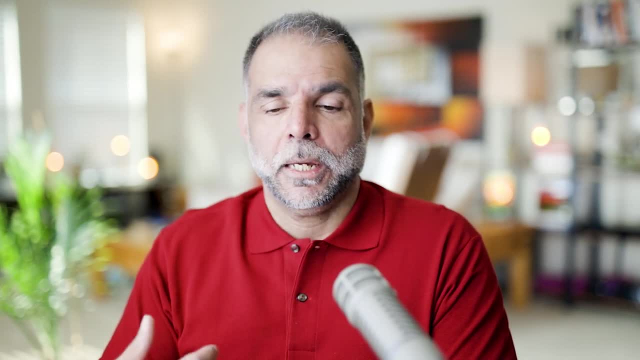 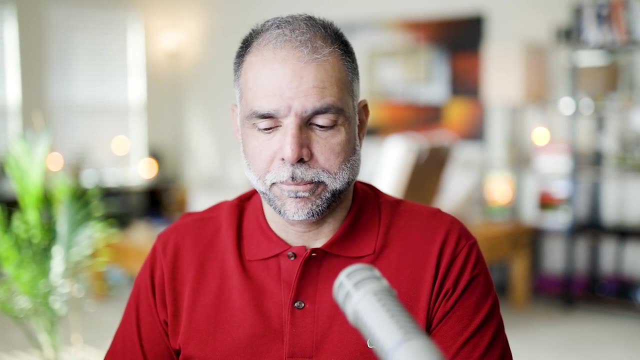 That partition key is something you decide And from that point forward the partitioning happens automatically by the NoSQL store. So they scale out rather than scale up. but they're built from the ground up to scale out rather than scaling up, All right. 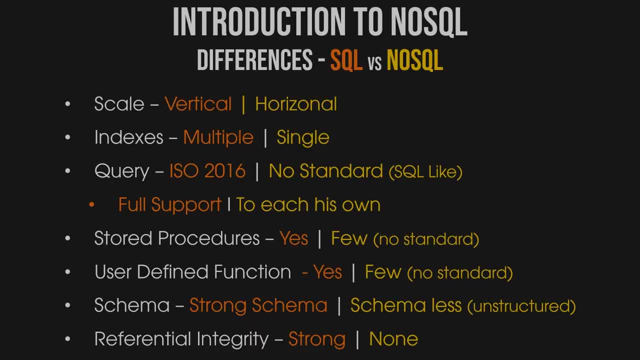 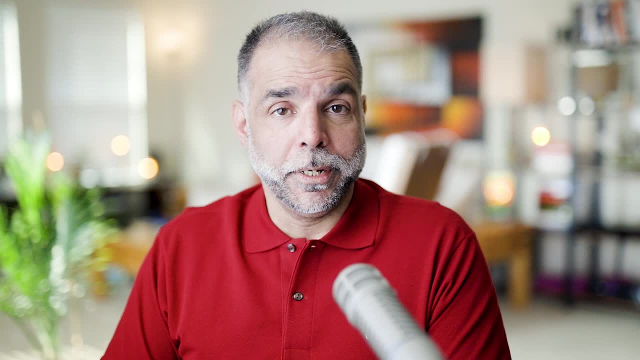 Okay, All right. So indices Now. there was a time where RDPMSs, of course most people know they can support any number of indices. NoSQL stores used to support only one index. Now they're supporting multiple indices, sort of a. you know mix and match, some do, and 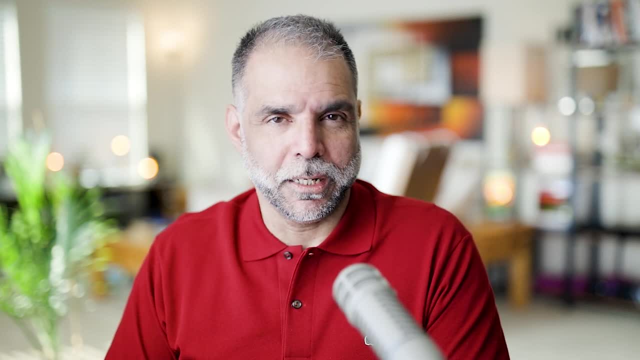 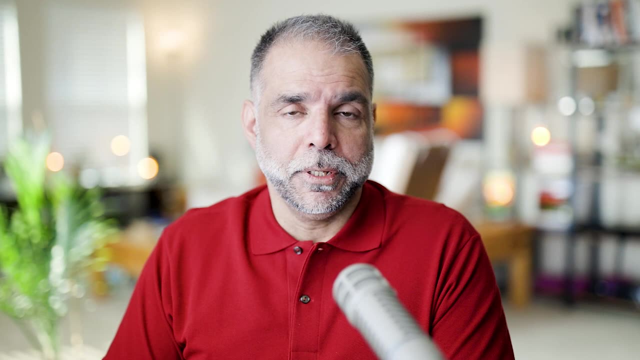 some don't. So I've just said single because for the most part that's kind of like how you want to look at it. There's truly kind of like this one index but you can have other indices like MongoDB supports indices on the fields inside of the document. 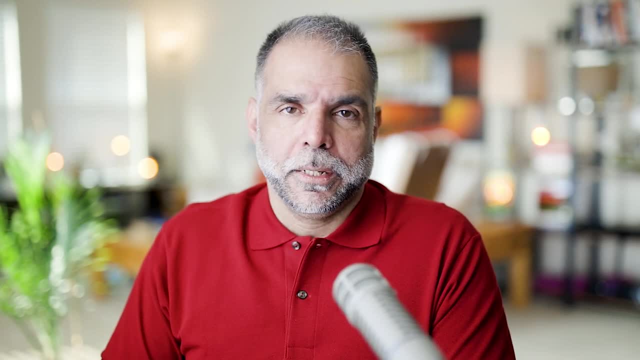 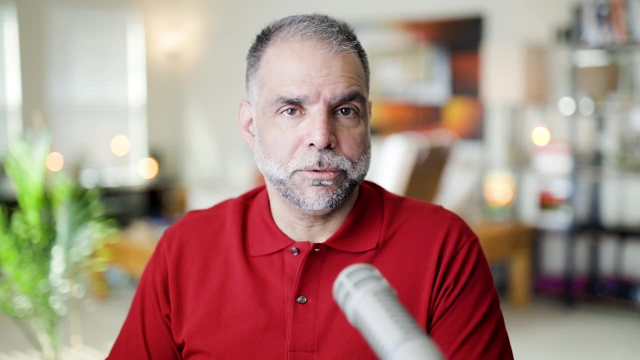 And so does CosmosDB. So it's difficult to categorize that. so I've just put single. but there's a difference, There's a limit, and that limit is based on the type of database- your NoSQL store- you're using. 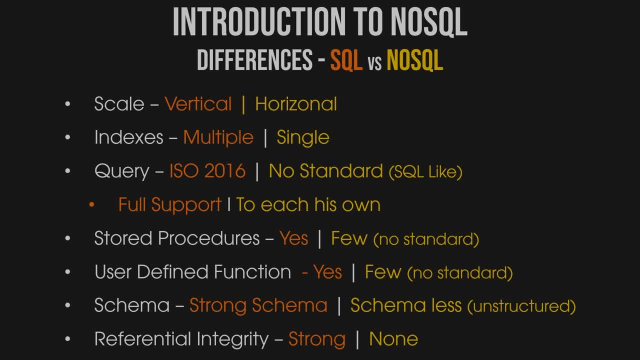 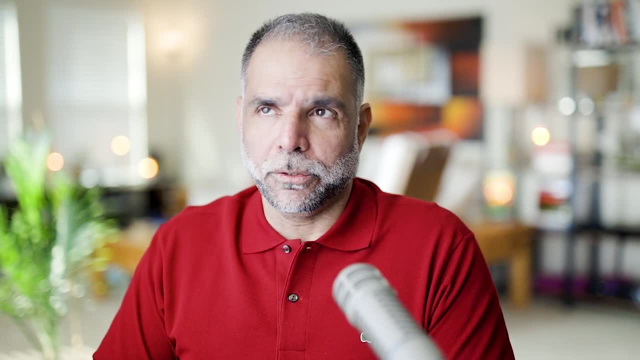 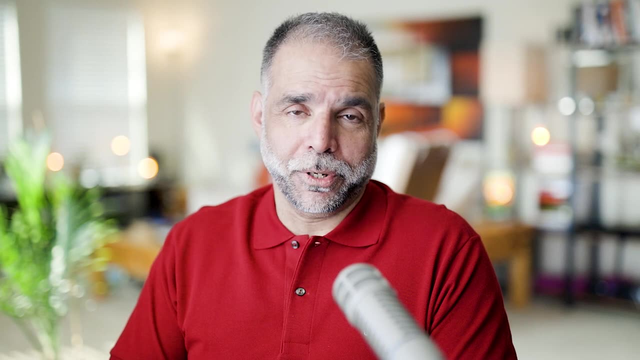 It's not common NoSQL started off saying it's NoSQL, then it became not only SQL And I used to wonder, like, so it's not only SQL, what else is there? Somebody says, I'm not only this, but then okay, you're not only that, but what else? 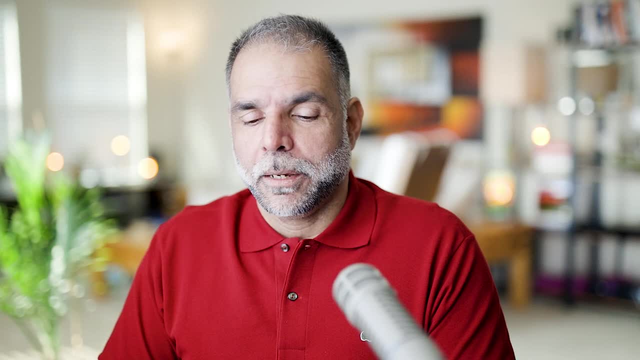 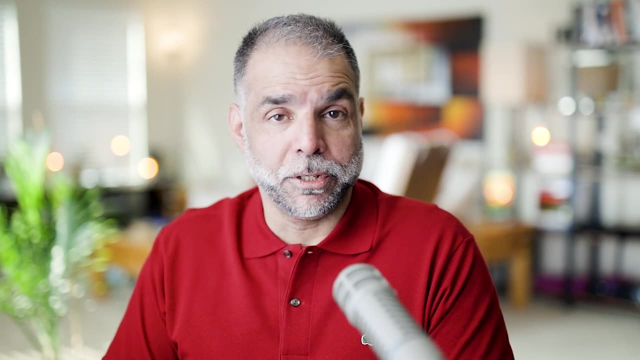 You know like, and there's no answer to that. Personally, I think that's a misnomer. this NoSQL store it's not NoSQL. it should have been No relational store, because that's what they really are. 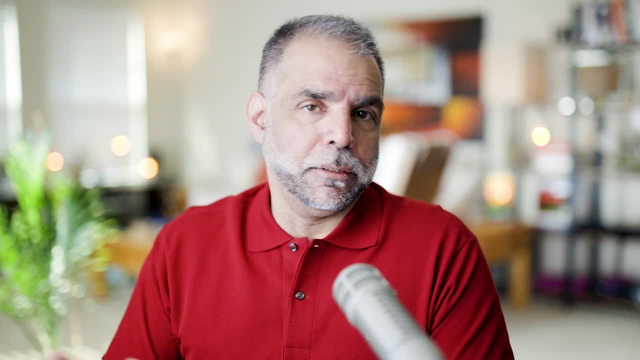 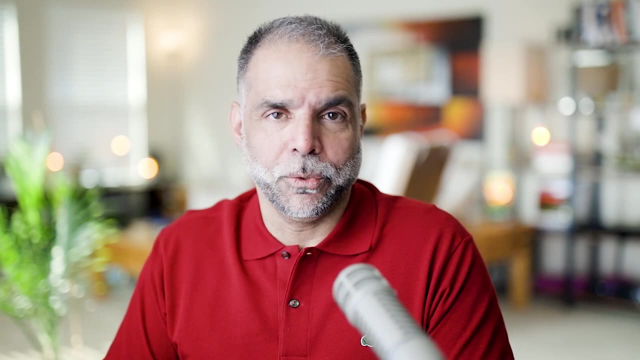 Most of them, all of them that, at least the one that I've worked with and know of, are non-relational data stores. It's not about the NoSQL, they're non-relational. They don't have the idea and the concept of relationships across, let's say, tables. 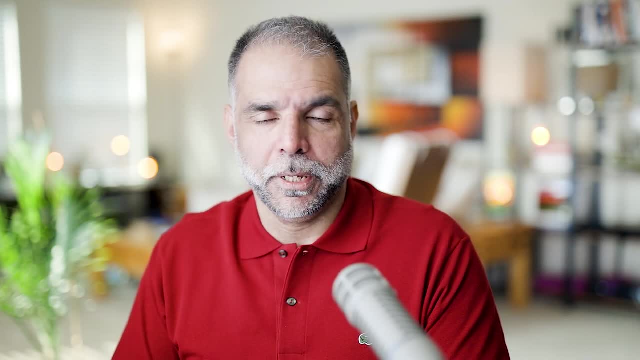 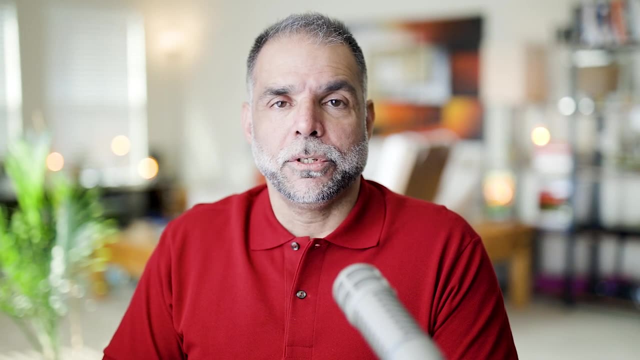 There's no built-in mechanism to support the feature or the database, The need for referential integrity and foreign keys and constraints across foreign keys and such. So there's no relationship. If there's a relationship, it's in your head. There's no relationship inherently built into these databases. 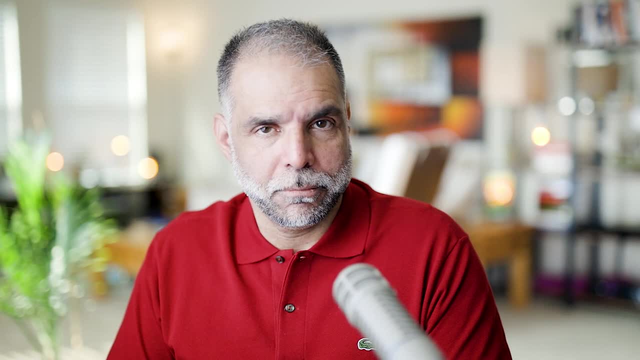 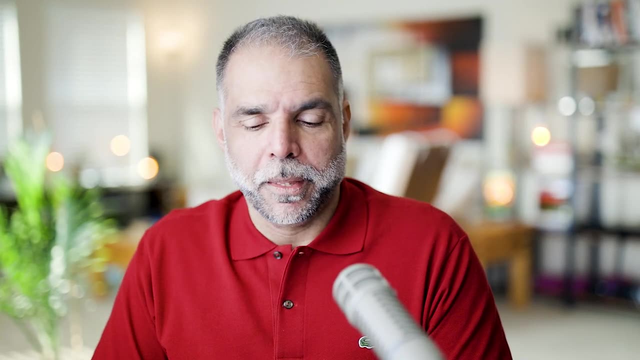 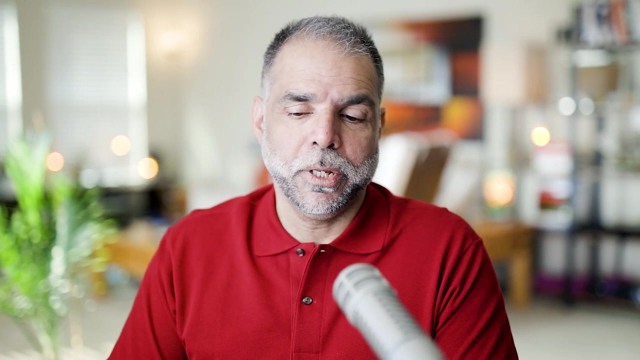 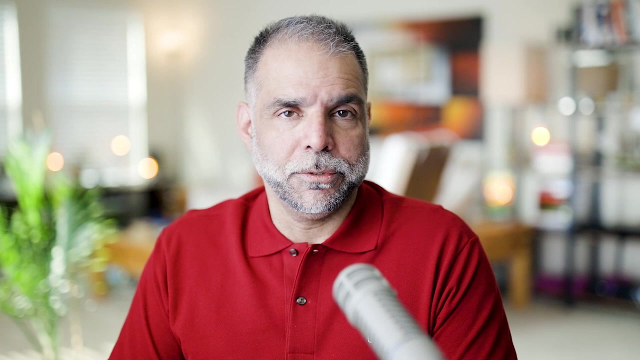 I think the right name would have been No relation databases, not NoSQL, But anyway it is what it is. So some of these NoSQL stores do support a query language. Some query languages are specific By them. for example, Neo4j, which is a graph database, has Cypher as their language. 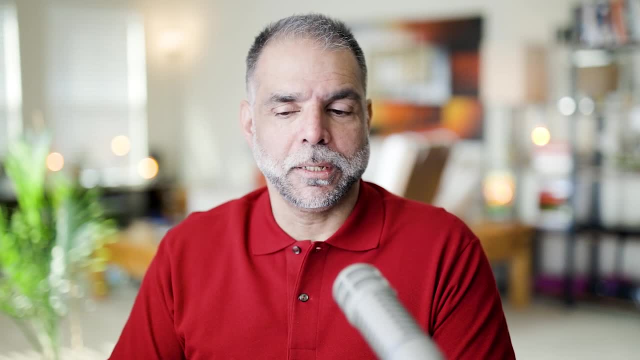 And then there's Gremlin, which is a more. both of them are open source languages, but I think Gremlin is picking up more traction And so many other graph databases are supporting Gremlin, So Gremlin is seeming to be like the preferred SQL language or dialect. It's not anywhere close to SQL, it looks like, but of course they're trying to do different things, So the vocabulary will be very different. Cosmos DB supports Gremlin if you're using the Graph API version of Cosmos. So between Gremlin and Cypher. these are more for the graph database aspects. 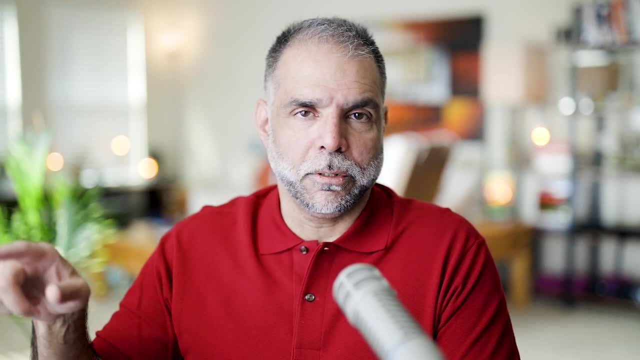 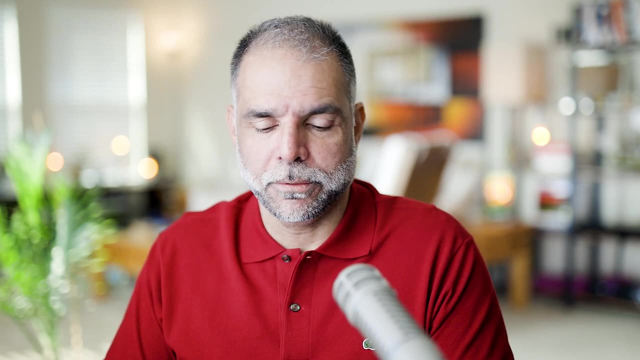 And I think Gremlin is more like a fluent syntax, you know, dot, dot, dot, whereas Cypher is more like an SQL kind of syntax. you know, just like we are used to using SQL and RDBMSs. Each has their own dialect. 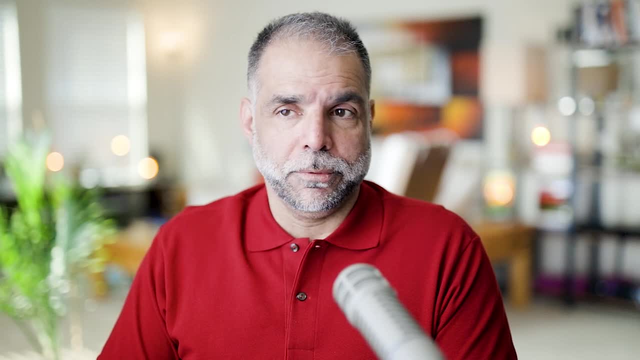 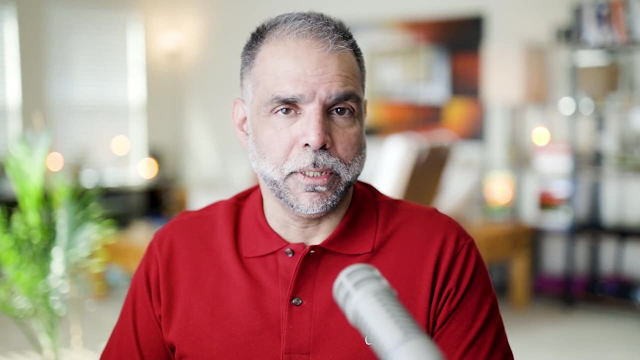 Each has their own understanding of what it supports And some keywords also, you know that mean something to us in RDBMS worlds, will mean or do different things in an old SQL store. So it's a crapshoot. I think at some point- maybe another 10 years, 15 years- they'll normalize to this one language. 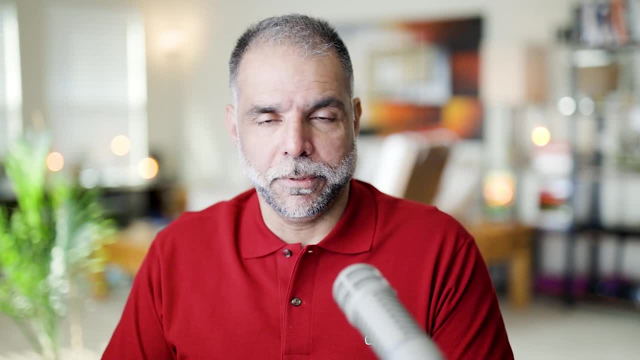 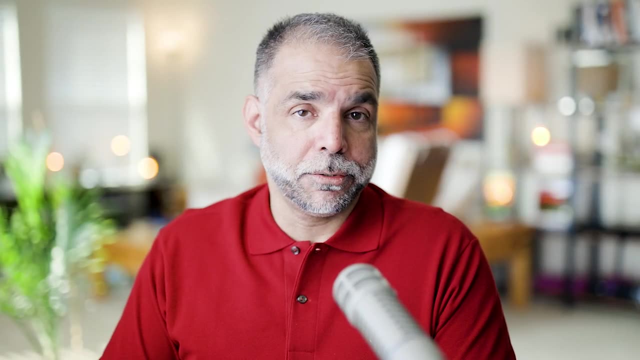 and there'll be some standards, But for now there's no standard. Each database vendor supports their own extent of SQL, but it's not SQL in that sense because, again, they call it SQL. they're trying to get there, but they have slightly different. 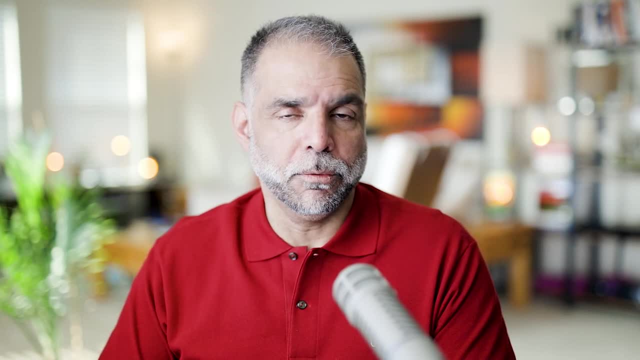 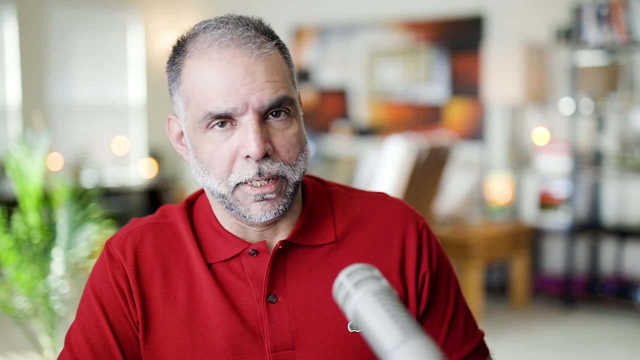 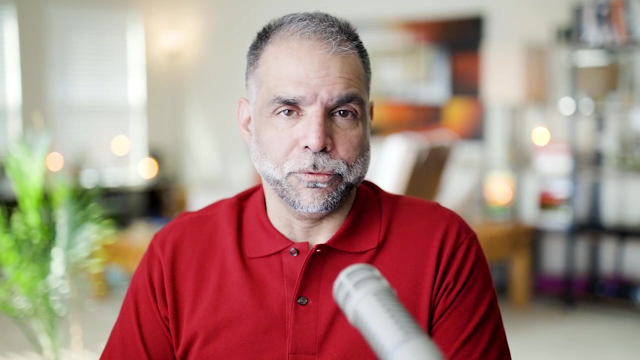 meanings for certain verbs: SQL words: verbs: right. So it's there, but it's fairly limited. No SQL stores, but I don't have it listed here. No SQL stores don't have the notion of joining, for the most part, right. 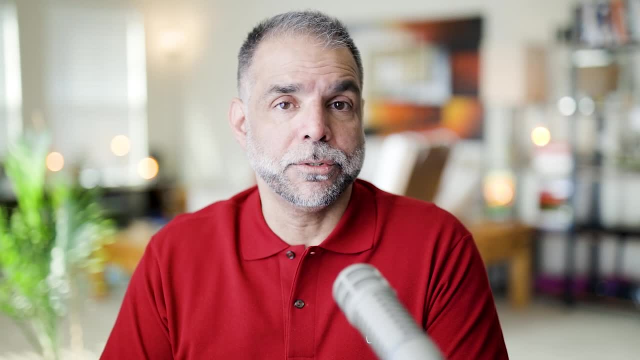 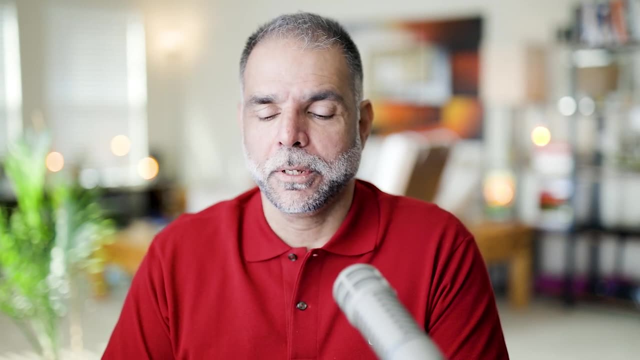 So the joining is something they don't support, which is why I said there's no relationship feature in the no SQL store. it should have been called no relationship or no relation. non-relational store database Joins. it's not like they don't support it. 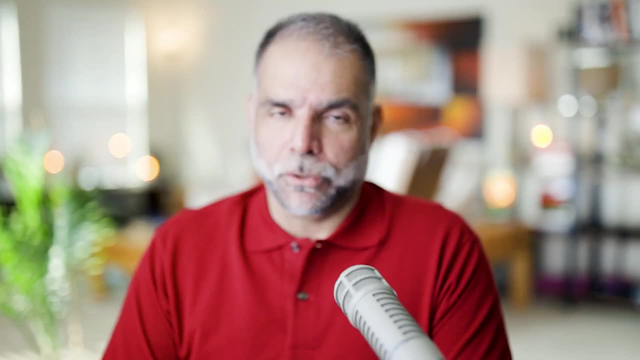 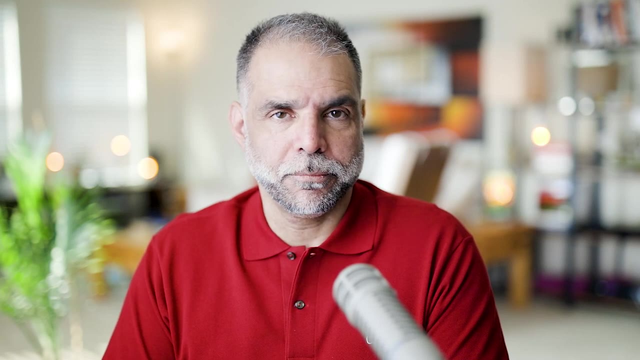 Well, you could do the joins by yourself in your code, right? They don't do it Now. maybe in future they'll even do that part, but for now they don't support the notion of joins and the notion of relationships across containers or tables, whatever they want to. 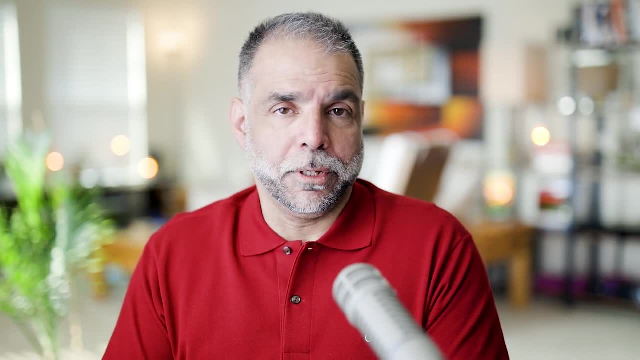 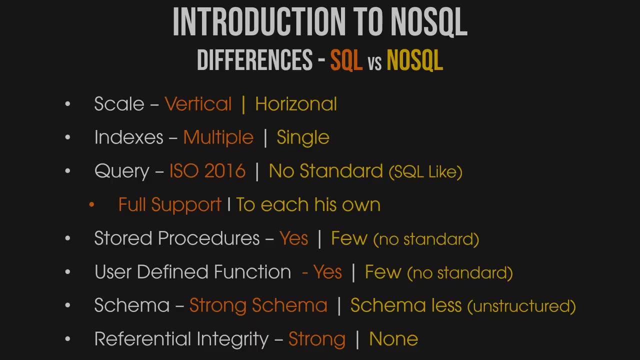 call that. So, as a result, the query languages have slightly different meaning. you know when you there's no notion of join in these languages, but there are differences. Okay, So now I need to go back to the end game and try out some more of the tools. that are all. 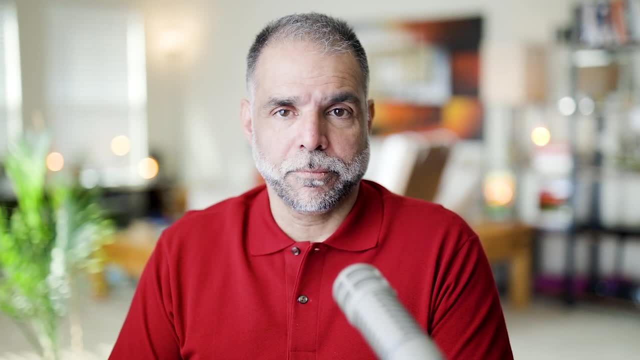 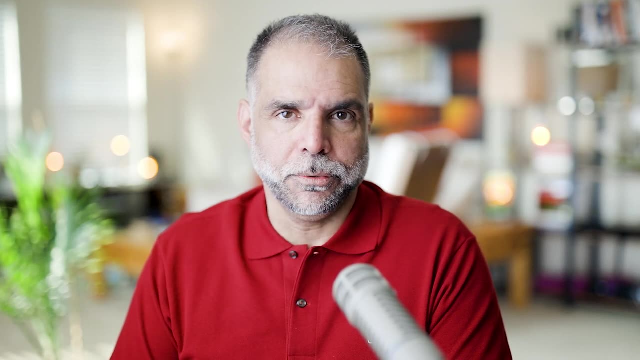 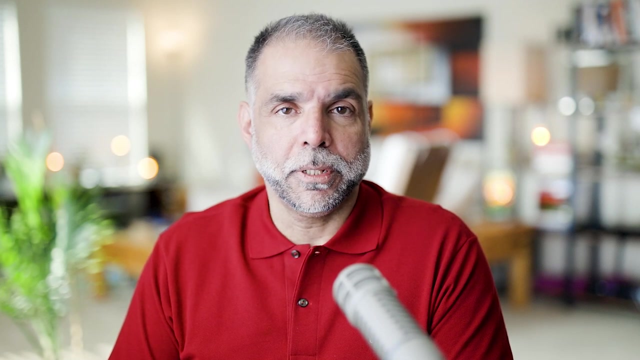 different. Let's try again. Let's start with the DIY type fields. So, JSON, we're going to find the lower end. So this is what you'll see here. So we're going to work on this one. We're going to talk about something called CI. 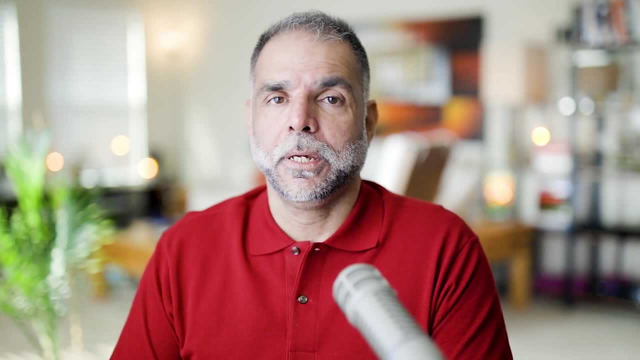 We're going to talk about JSON, which has a very interesting concept. What is this? The CI. it's a very interesting concept. It's a very interesting concept, a very interesting concept to talk about. There are a few things that I want to talk about today. 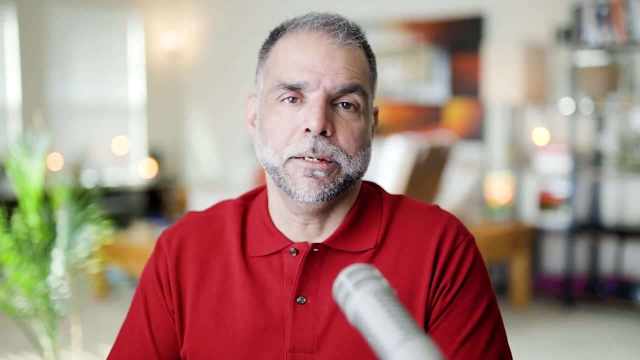 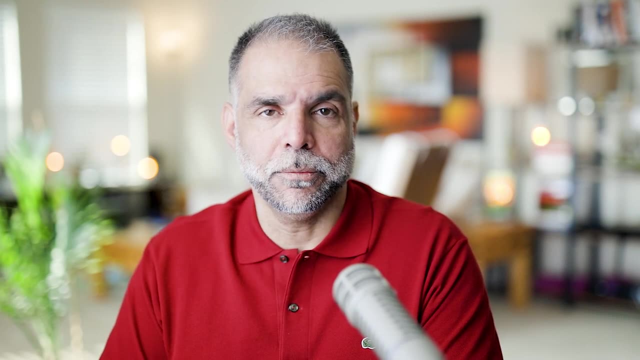 There's the, for instance, the colon have these ideas, but they mean slightly different things, so they can do slightly different things, or there may be limitations with what they can do versus what you're probably used to in rdbmss. so even though they're there, they're different. 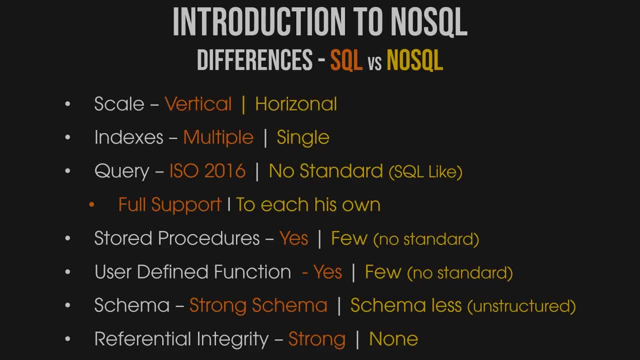 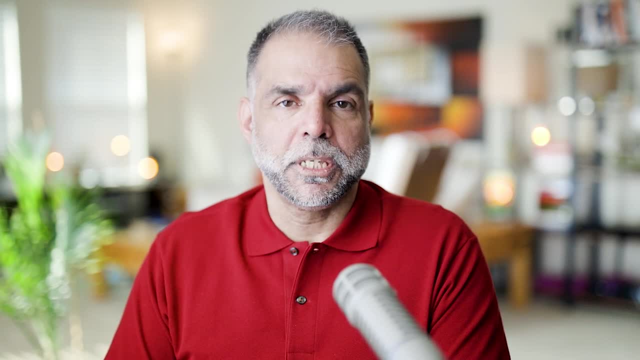 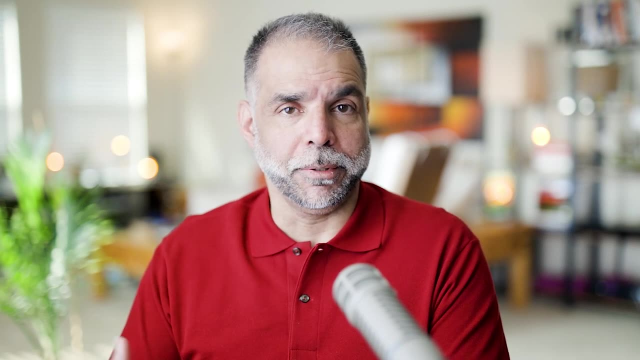 of course, rdbmss are strong schemas and no sql data stores are schemaless. schema agnostic is probably a better word for it they're. they're agnostic to schema, the schemas in your head, the schemas in your application. your application code might be aware of the schema, but the database 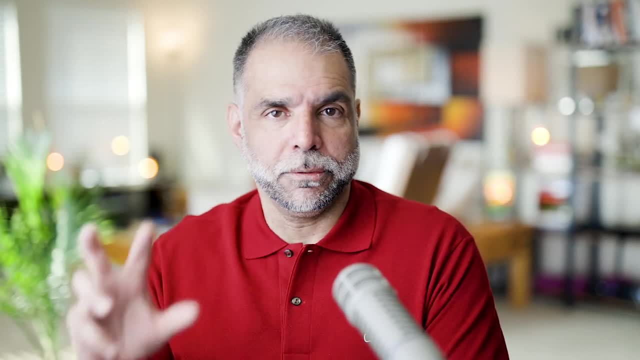 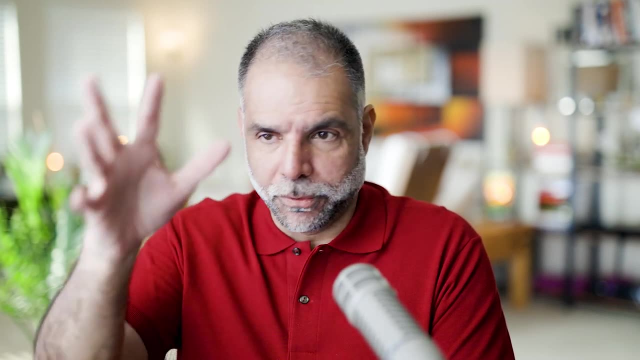 itself doesn't give you the option to specify schemas or define data types for columns or any of that nature. you can put what the heck you want in every record in your mind. if you want to put this in this container, you want to put only customers here? that's up to you, right, but it's. 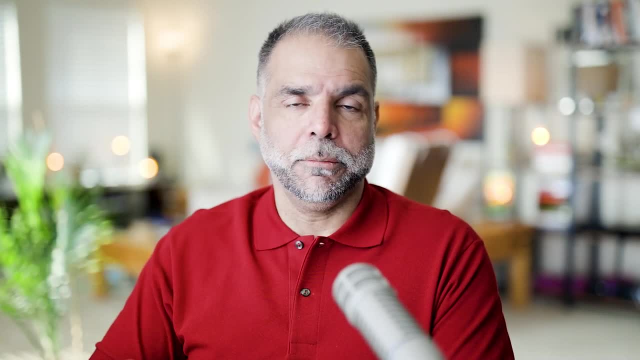 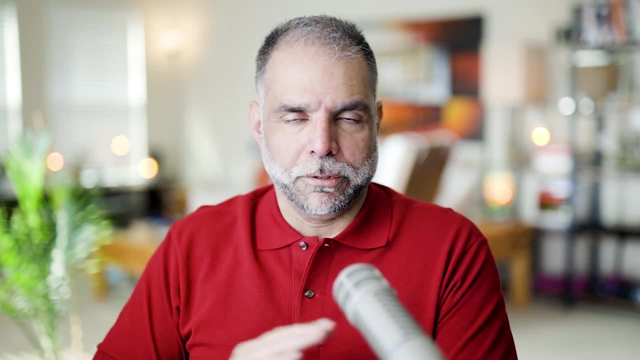 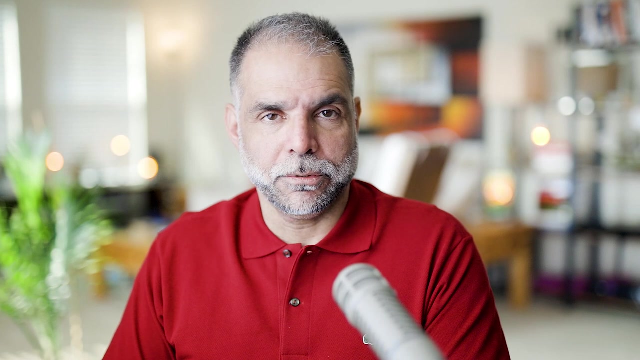 not like it's required every record in a no sql store database for this white column or document db or cosmos db- i'll talk about that later. you, they all support this idea that every record can be a completely different schema. so the schema is something you control at your application. it's not determined or controlled by. 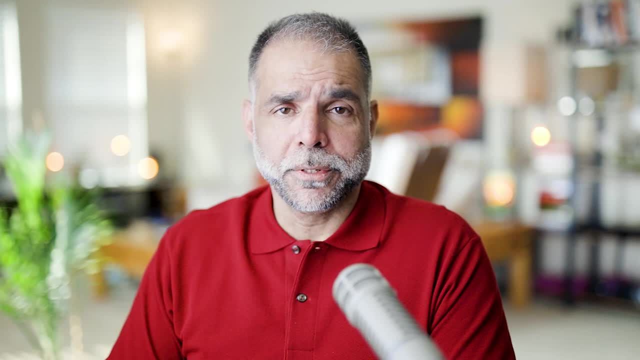 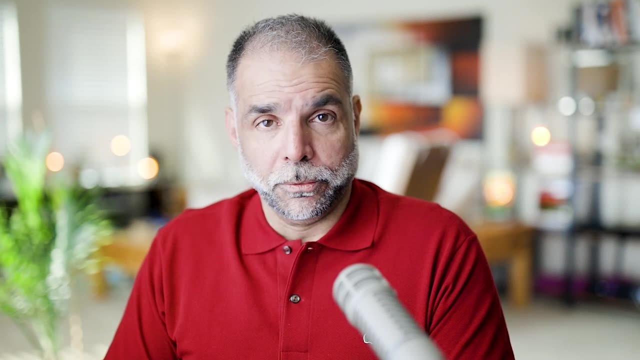 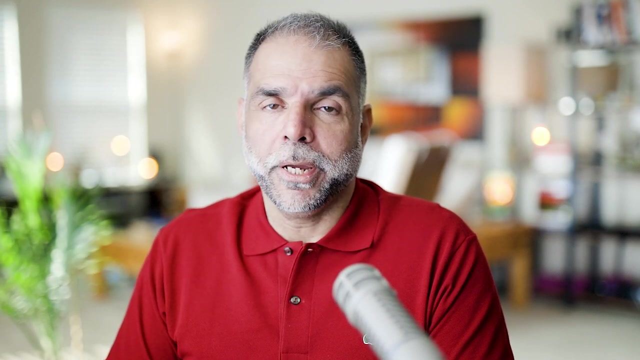 the database. now, that is one of the reasons that no sql stores became popular. there are many businesses, imagine like the facebooks of the world or the googles of the world, right there. how do you model a database for something like facebook or even google, but you don't know where? you're headed right. it's like every day is a new feature you want to add on. now you need a whole other set of tables to support this and relationships with pre-existing tables, and it becomes a nightmare. in other words, that strictness, the schema and relationships and differential integrity and all that is coming in. 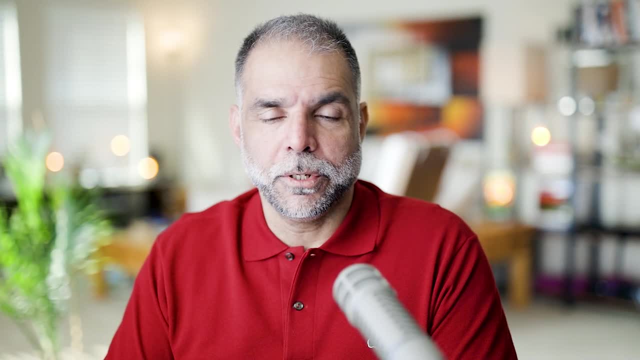 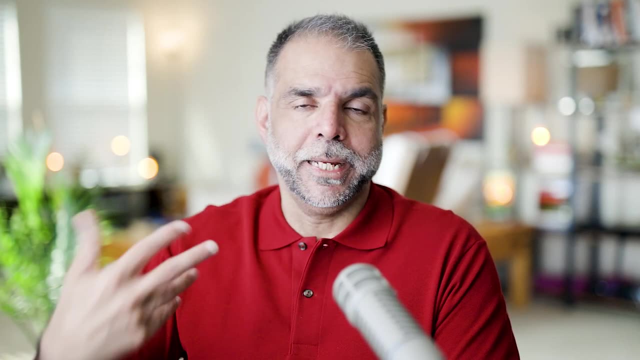 the way of you being able to progress and move faster. so in many ways no sql stores are beneficial to those businesses that have that need, but suddenly one day from the next you're going to slap on new data and forget relationship and i don't know. care for the scheme. i just want to. 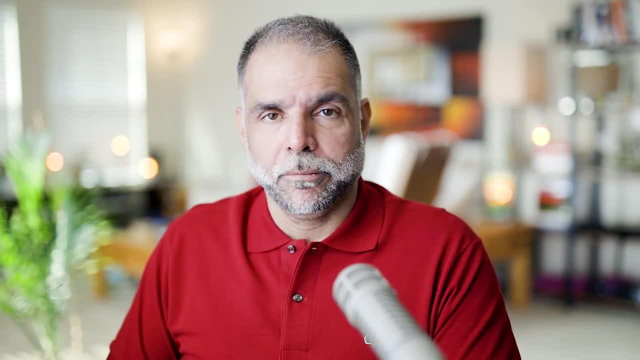 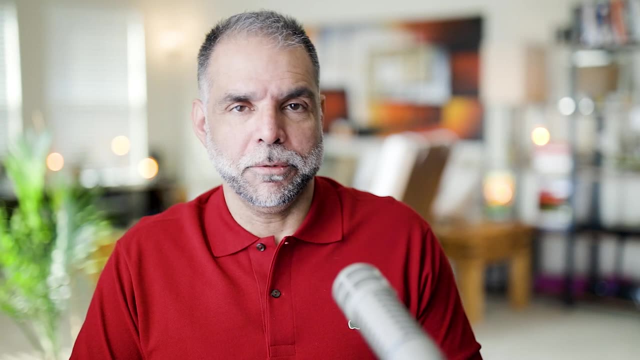 capture all this data right, big data, machine learning. these are areas where you can't predetermine the, the schema. i mean, if you sat down trying to determine the schema for every one of these scenarios, you probably won't even start writing the code, because you'll just be building. 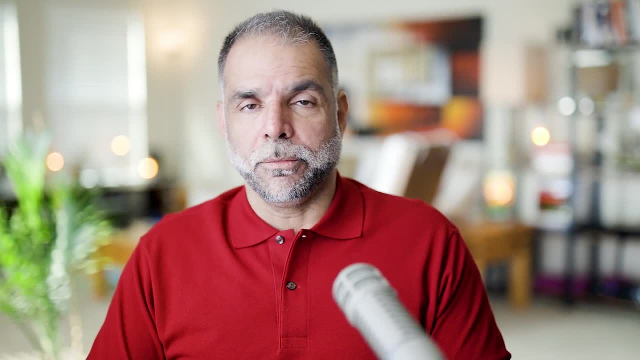 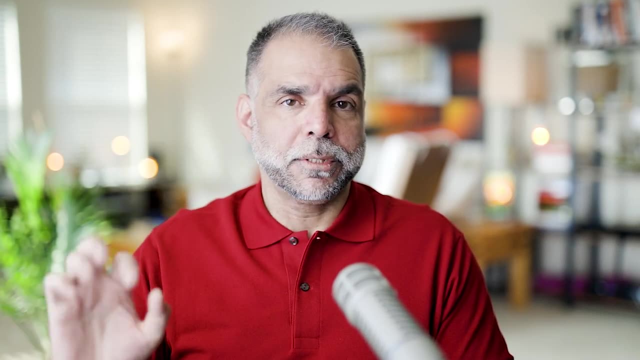 out these schemas, so no sql stores- support are really good for those kinds of businesses where maybe within your business there's a certain component of the data that is schema less and that might be useful for you to use no sql stores for that portion of the data because it 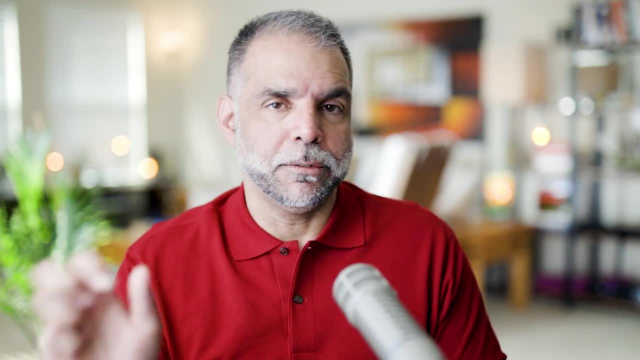 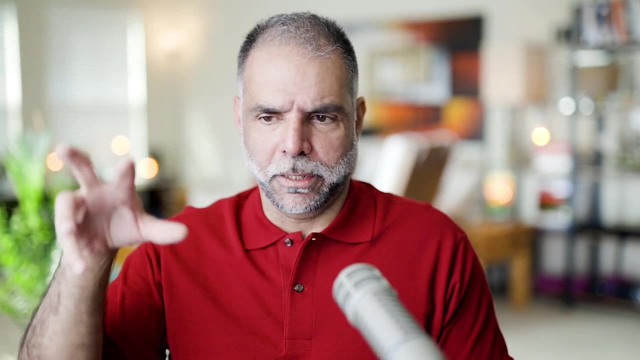 just allows you to sort of store the data, still be able to retrieve it and indexes and and do the analysis and whatever. but it's not forcing you to define a schema up front and stick to a certain schema. whether can this field have to be there? i don't know if everyone is going to give me that. 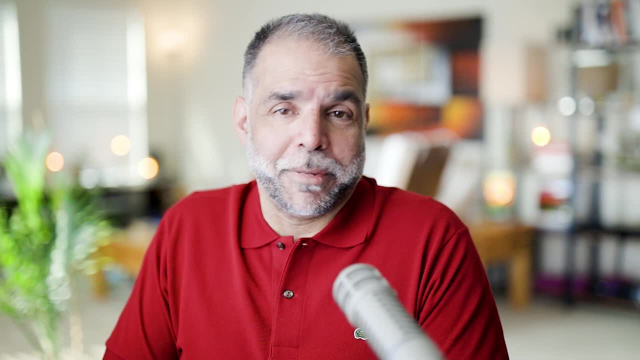 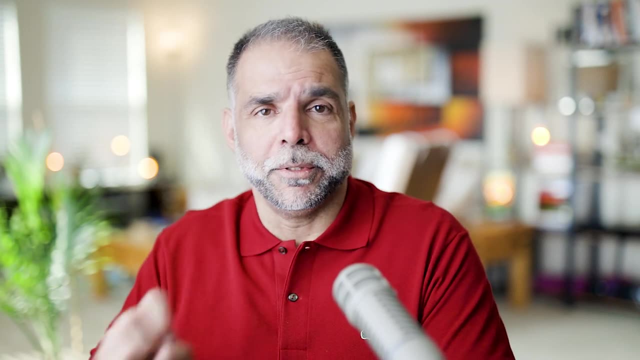 field or not. i mean, i'm not even talking to, it's not my business in the sense that i can't control it right. there's data coming off the internet, social media. you can't constrain people into saying you must provide me this field and that field all the time. so no schema databases and 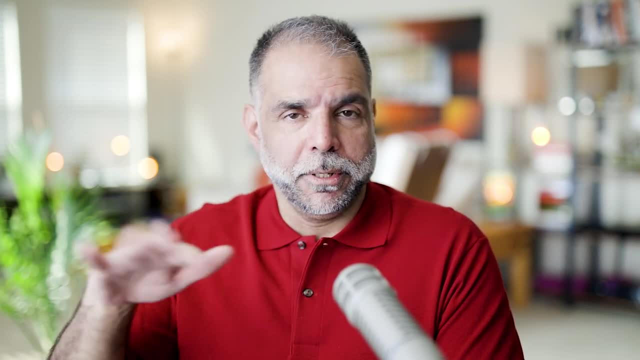 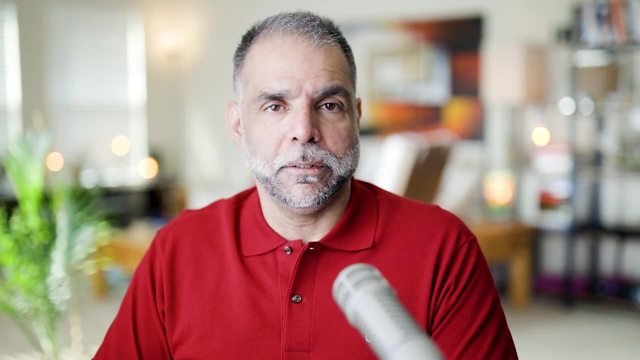 that's the reason. no sql stores were very popular or became very useful. during the same era, same point in time, when amazon and facebook and twitter and linkedin- all these social media websites- were kind of getting traction, graph databases did the same thing. graph databases also started to take off, doing these. 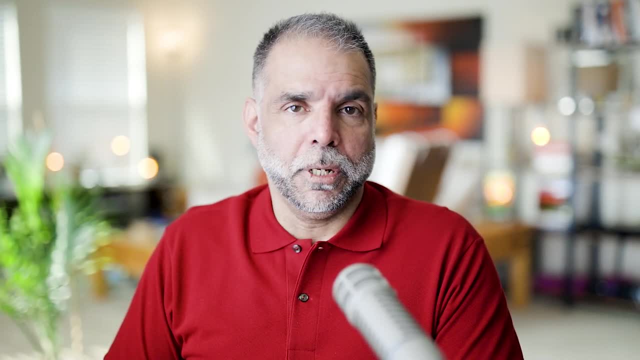 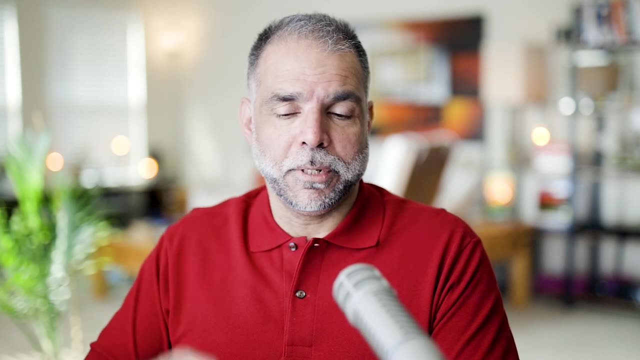 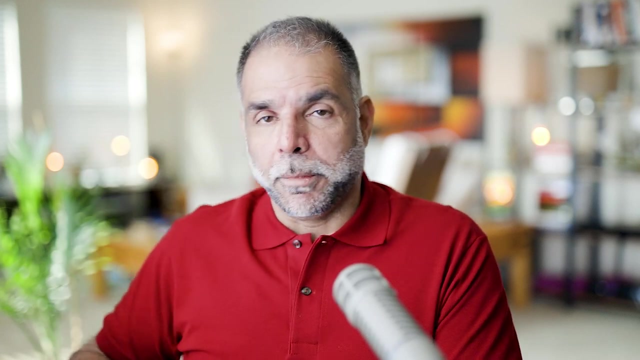 because social media are one of the larger consumers of graph databases, because they can do all this other analysis and find relationships that you can't imagine existed and typically relationships that are not only you know, so many degrees of separation from the original. you know, let's say, person, but coming back up from somewhere else to the person that 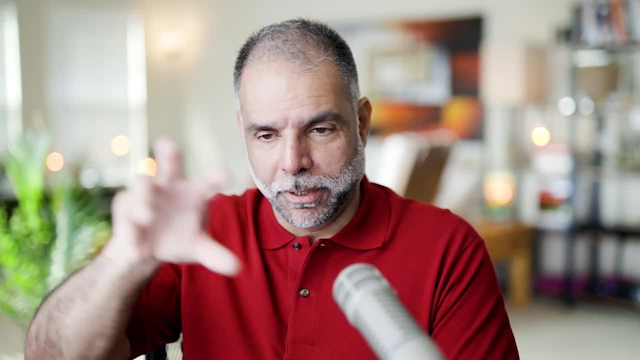 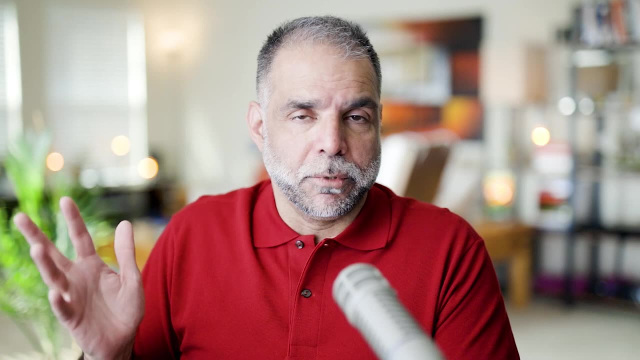 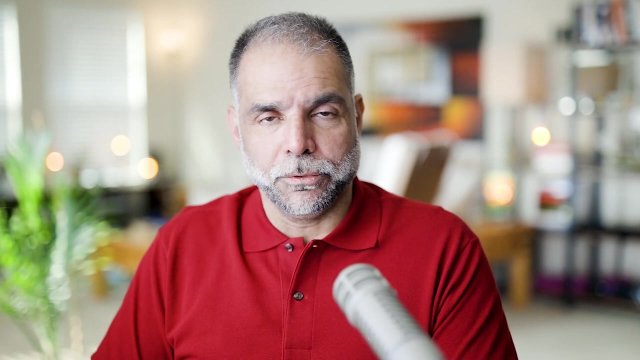 you're talking about. so you, you might see one relationship going from person a to b, c, d, e, f, g, but then g might actually have a direct relationship with a. for some other relationship come- not anything to do with this graph, so anyway. so both these new graph databases. 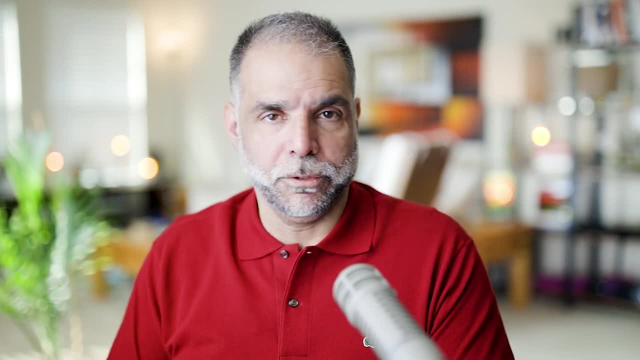 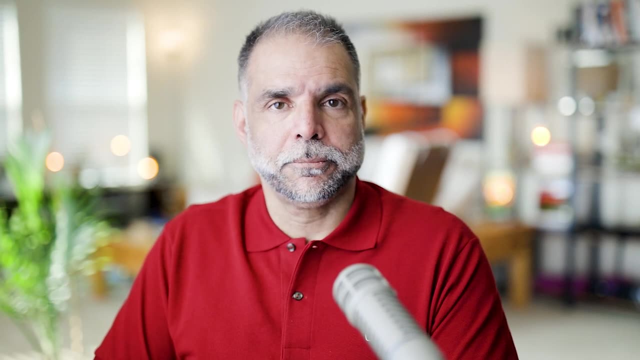 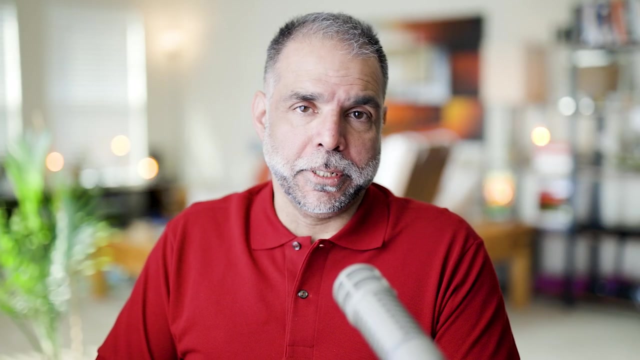 and no sql stores started to kind of gain traction during that time and there was, like this boom of internet, large companies like facebook, you know, and twitter and linkedin kind of taking off. okay, referential integrity: in rdbms: you can define what you want, it supports it. the database engine: 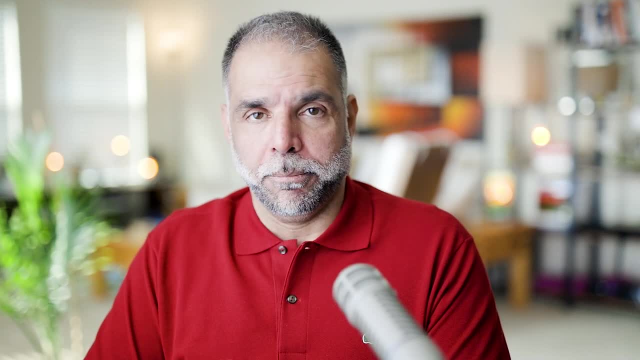 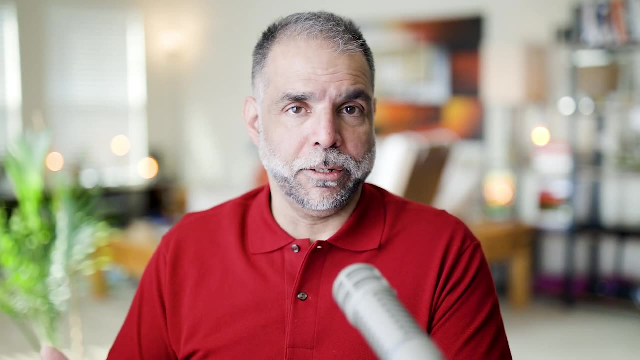 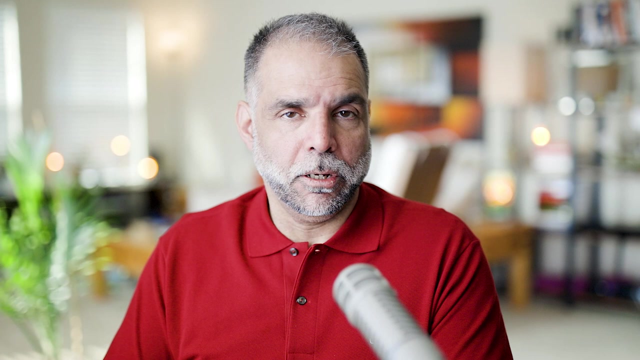 manages the integrity of data. the purpose of the way you define your data model in rdbms is also is by way of normalization, which is it's the whole intent or purpose is to remove redundancies, meaning duplications, and to prevent, update and delete anomalies, which is you know. 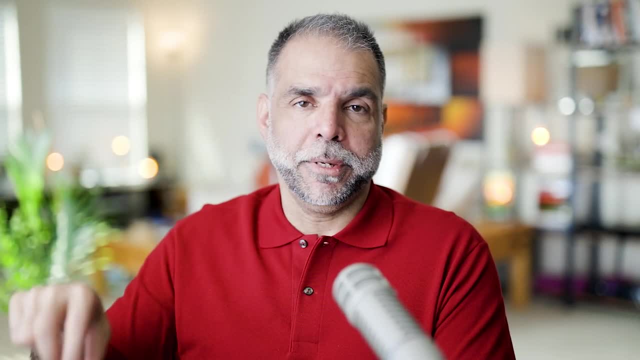 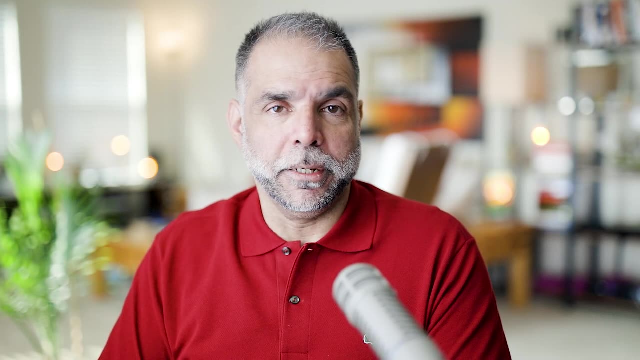 like if you have. if you duplicate data across your tables, then you make an update to one area. you have to make sure you update the data somewhere else. so that's the update anomalies, in case something has not been updated. it's kind of out of sync- and the delete anomalies are the 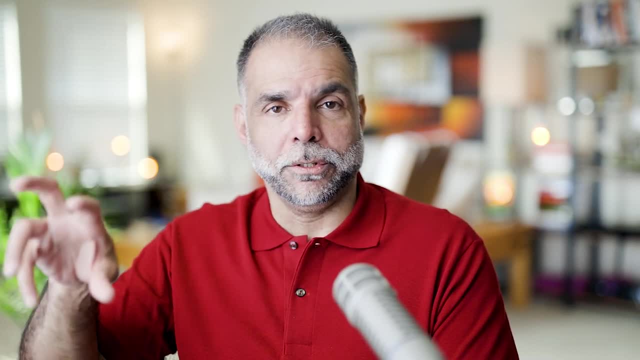 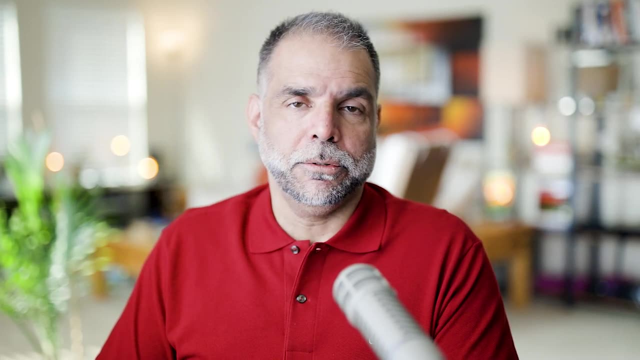 same if you duplicate the data in multiple places and you have to delete this one thing to make sure you delete it from other places. so the idea of normalization is, of course, to ensure that you don't have the update anomalies, you don't have the delete anomalies and the referential integrity is. 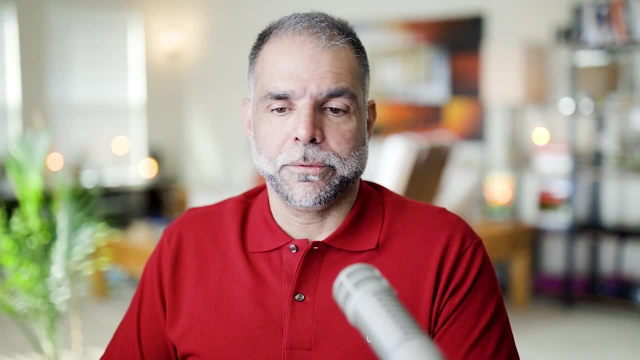 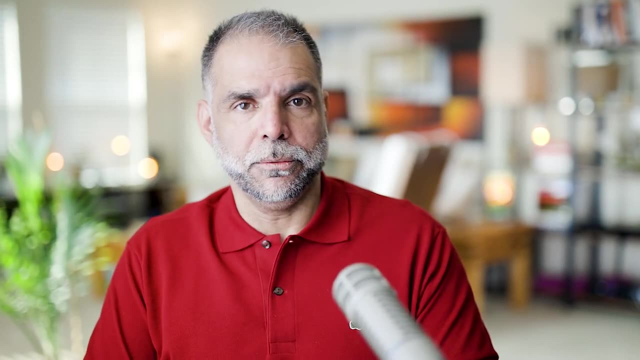 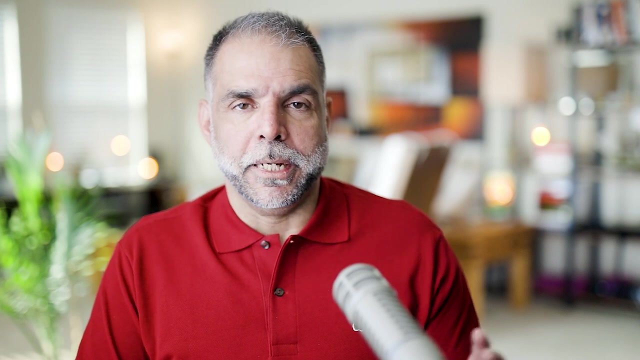 not a part of that. in no sql stores there is no notion of referential integrity. so one of these ways you want to look at no sql stores as compared to rdbms is this: whereas in sql stores, rdbms is the database engine is responsible for maintaining the maintaining your integrity. 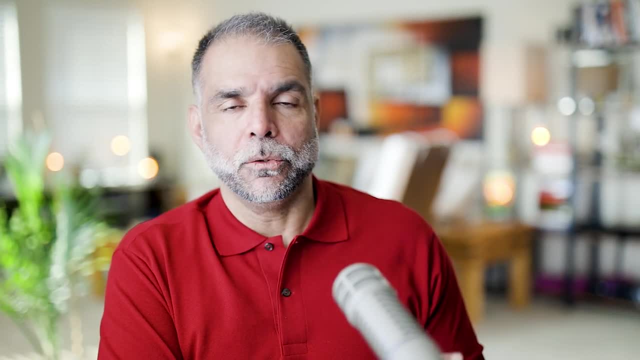 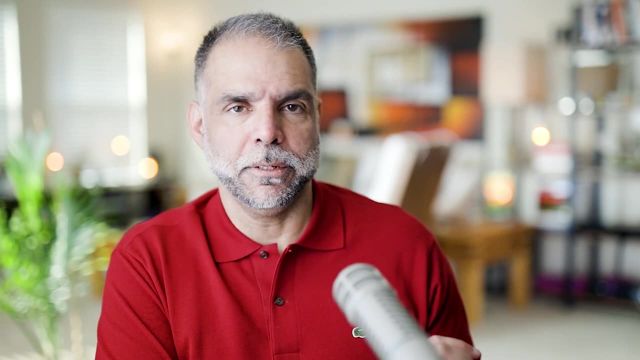 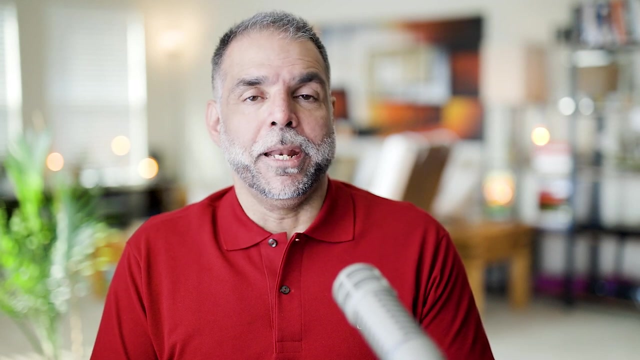 maintaining the referential integrity in a no sql store. if you're using a no sql store where the data has notions of relationships, which is very common, right- most of our business data is relational in some way. it is up to your application code to maintain, to manage the integrity and that might not make sense. but 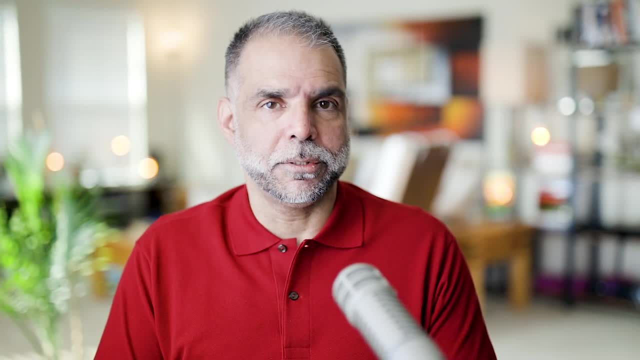 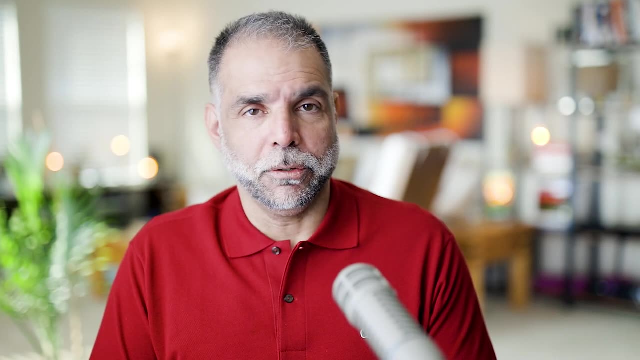 i'll just go a little bit into this and of course, in the next videos we'll go a little deeper into understanding this idea. whereas in an rdbms you're dealing with, you're starting your data modeling and doing a normalization, which is you're removing the redundancies, you know you've got foreign key. 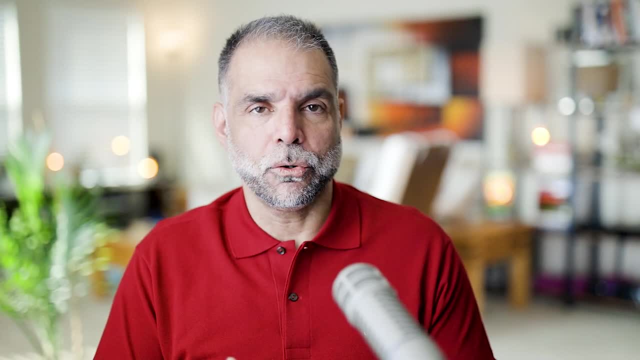 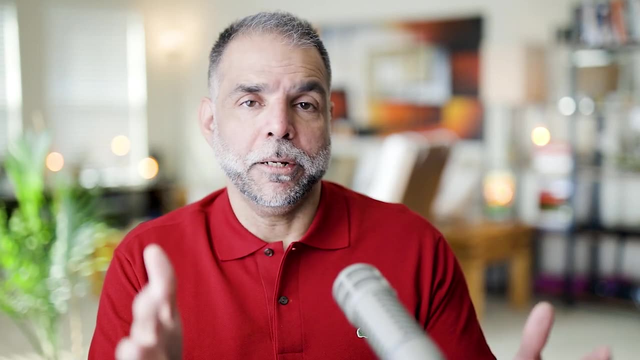 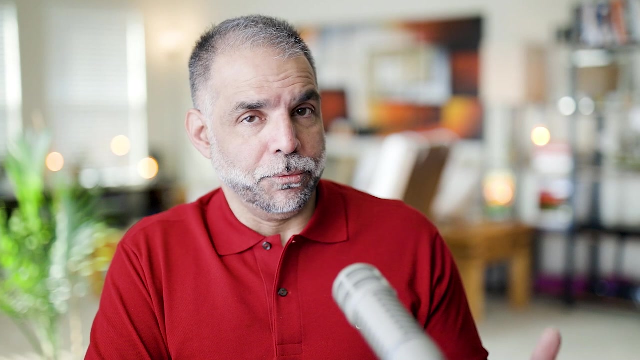 relationships, you've got constraints, all these things to ensure at any point in time when the data goes into this database it is correct and clean. and then when you pull out the database, you typically have views that do all the joins right and the database engine manages all of that for you. you know, gives you. 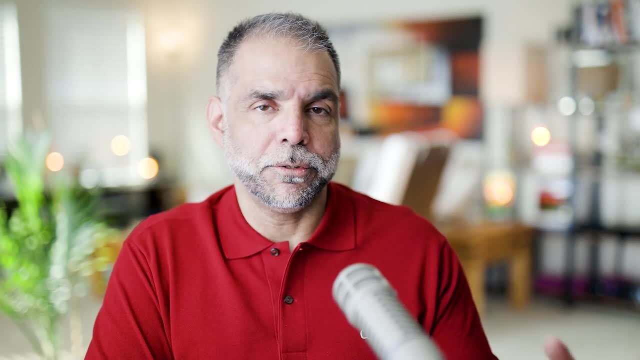 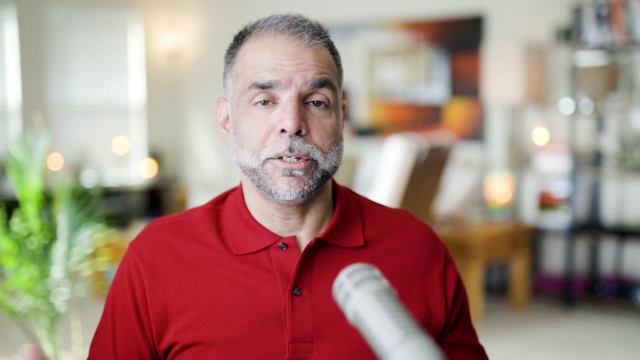 good query engine as well as maintains the gives you a good referential integrity engine. let's say you know that manages your indices and foreign keys and constraints, and what have you to ensure the data that goes in, no matter which application puts it in there, is clean and correct. 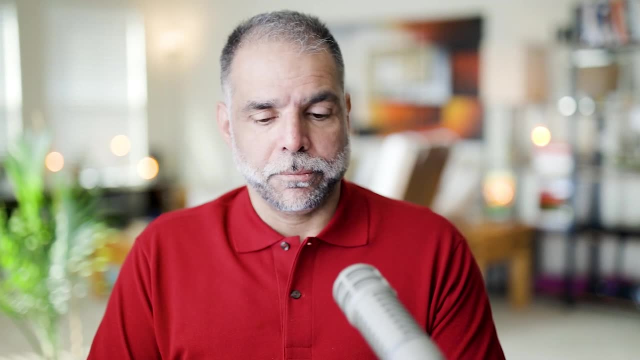 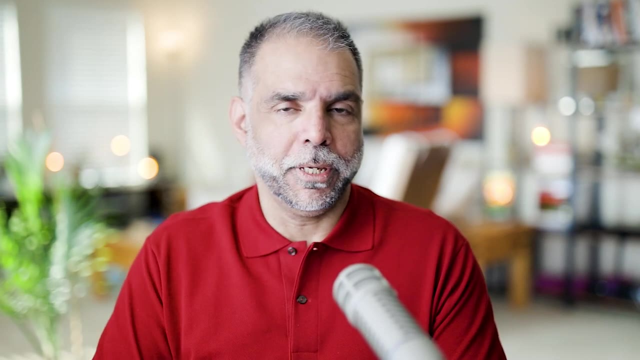 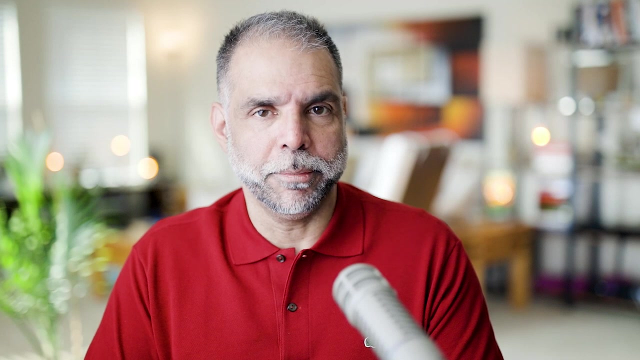 in a no sql store there is no such thing. so the onus of maintaining the integrity doing queries. of course now we have, you know, engines nowadays that have some some support for query, the decent, not nothing like an rdbms, and i'm sure that over time they'll get better and better. 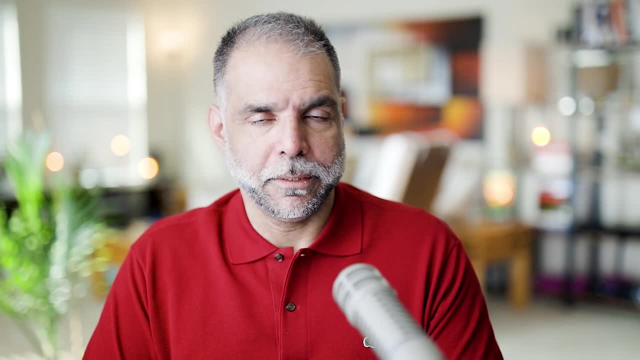 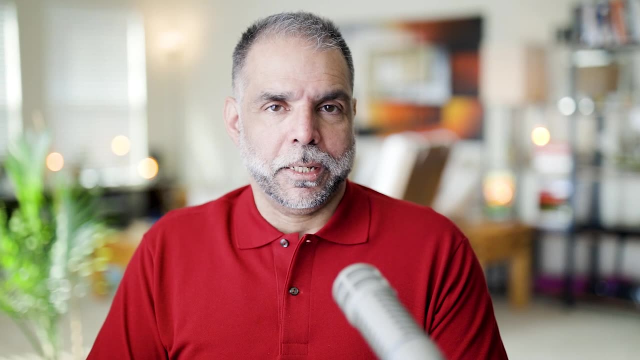 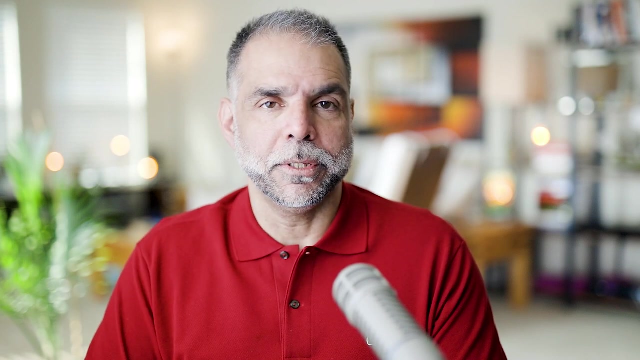 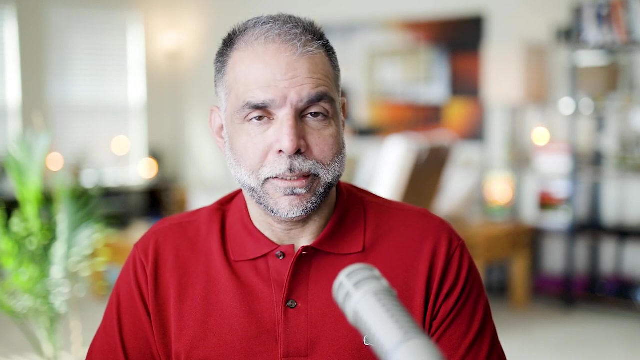 but the referential integrity idea that rdbms has provided you, you have to build into an application yourself. now i'll tell you why that happens: because in no sql stores you're primarily not concerned with normalization. you don't care for removing the redundancies. in fact, most times you're duplicating the heck out of your data. 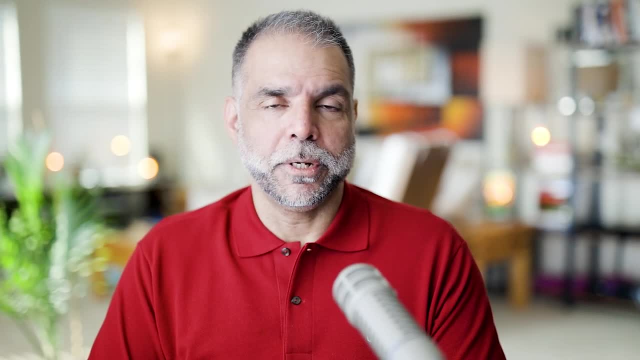 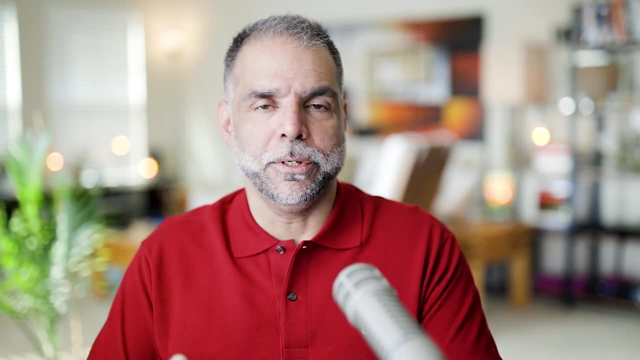 so imagine, in an rdbms when you create a view, let's say you've got these 10 pages in your application, for each page you got a view or a query that gives you that data right. does all the joins in a no sql store. you want the data to be saved in that fashion because you don't. 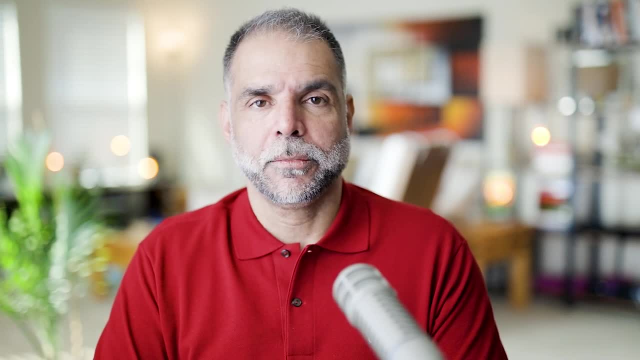 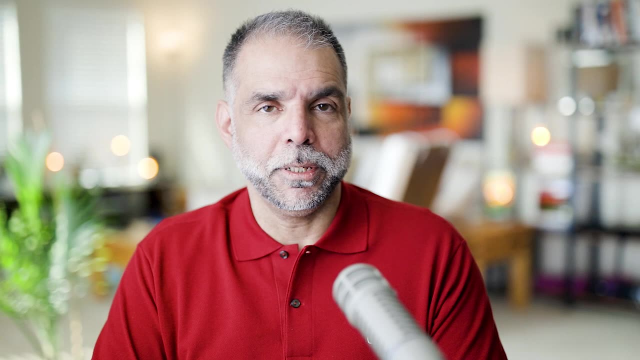 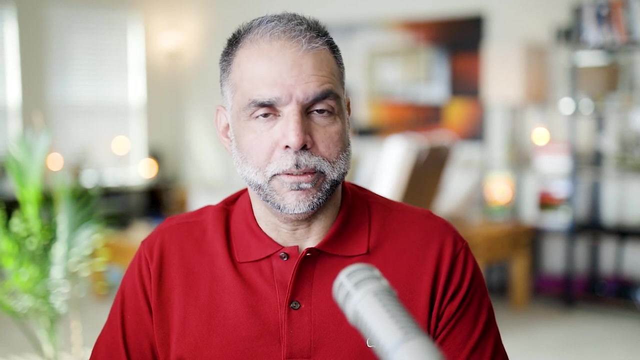 have these powerful query abilities. but if you did that, you've potentially duplicated data. right, but that's what you do in no sql store. now, that might be shunned upon in an rdbms world, but in no sql store there's no problem with that. but now that you've duplicated all this data, 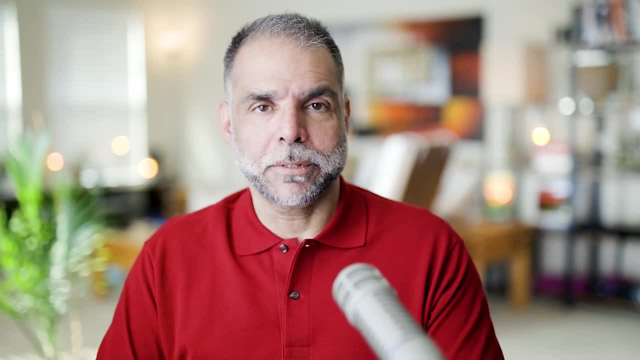 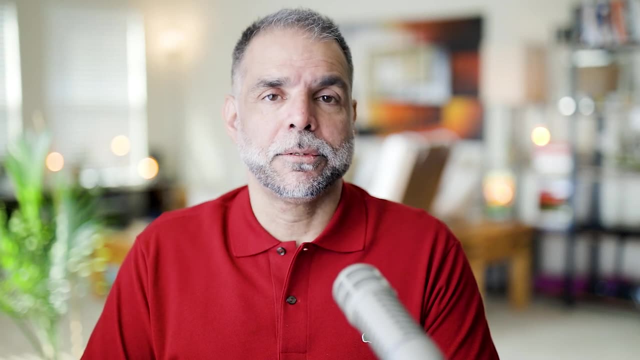 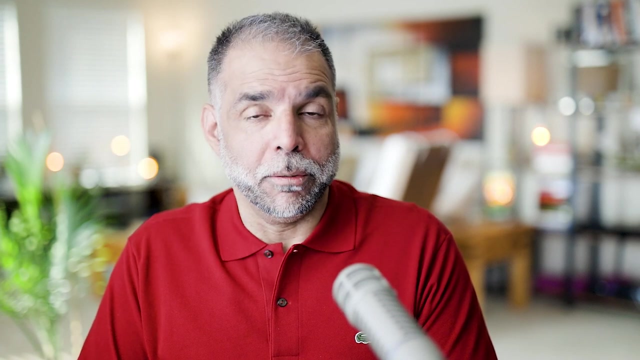 who's going to delete stuff when something gets deleted? it's scattered in 15 different tables, right, like, let's say, your customer data, then 15 different tables in your system, which is good, which is a good practice, but now you've got duplicated data. so who's going to ensure that there are no delete anomalies or 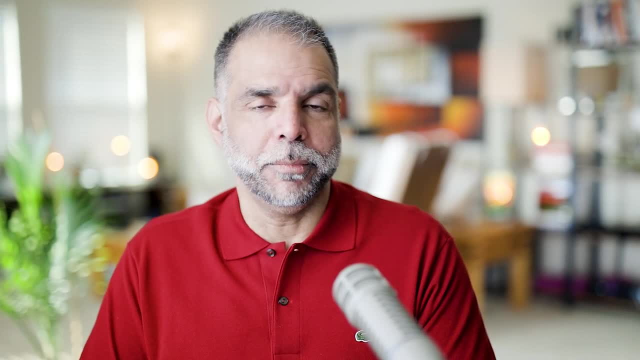 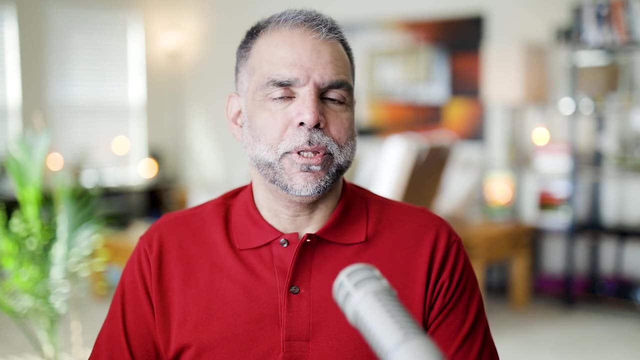 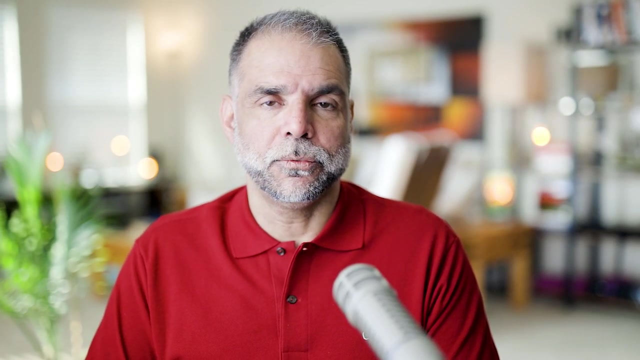 update anomalies. right, that's up to you. your application code has to maintain that or manage that. that's sort of the onus comes on you. this might seem like weird, and why the heck would i ever do that? all i can say is: if your data is such that it works for a no sql store versus a rdbms. 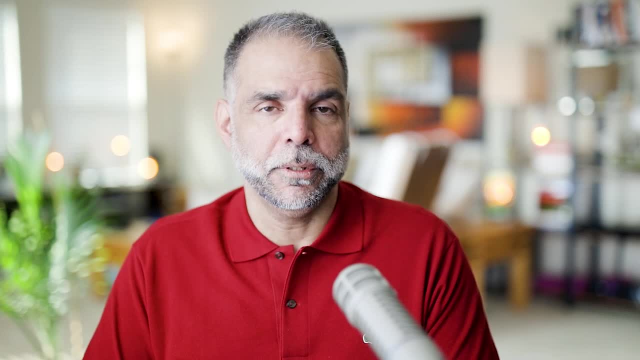 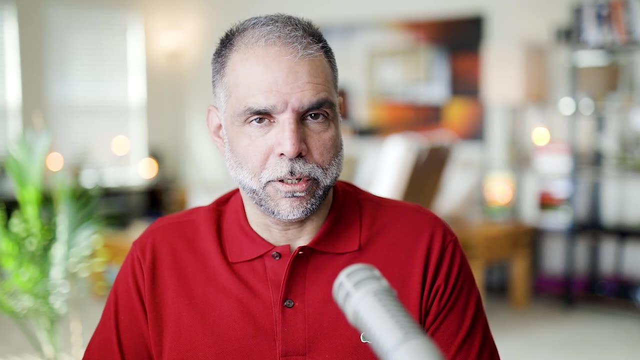 in terms of the schemalessness. if you will, you know the value. if it's purely relational, you're probably better off using an rdbms. if it's not, you're probably better off using a no sql store. that's not to say that you can't use or should not use. 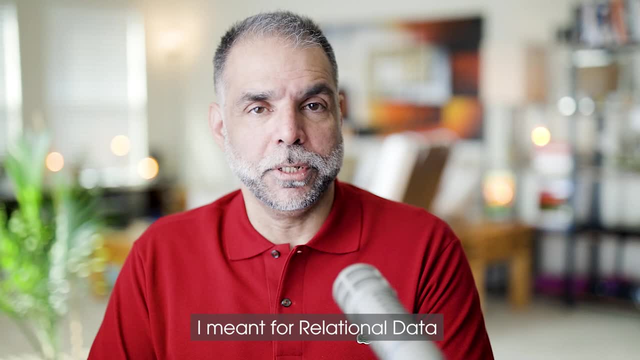 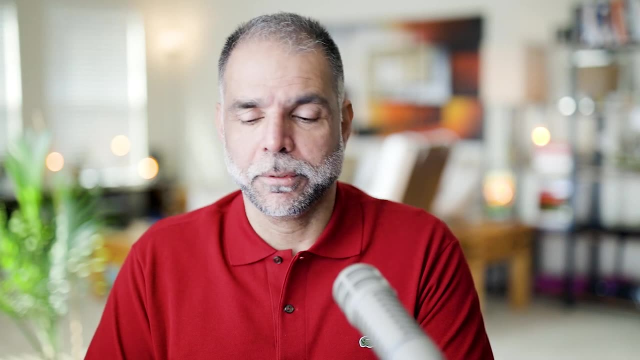 no sql stores for rdbms could mean that you need the scale, you need the horizontal scale out. rather sorry, horizontal scaling versus the vertical scaling or scaling out versus scaling up, this just depends. i'm not in this video, i'm not going to tell you which one you should or should not use, but i'm trying to just show you the difference.